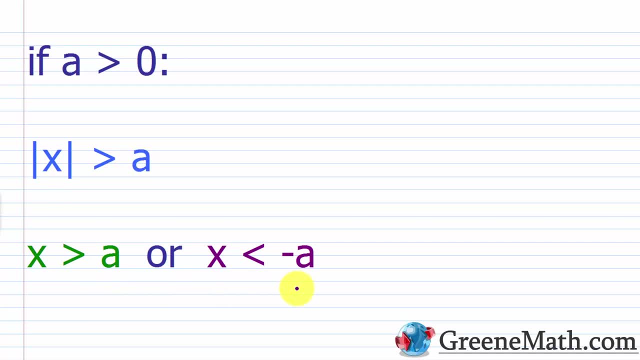 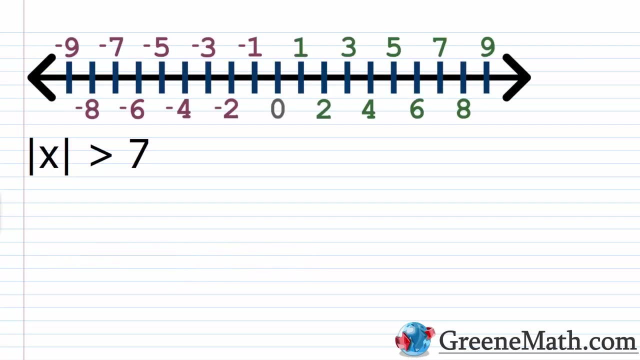 real number. this gives us an or right, a compound inequality with or. so x can be greater than a, or x can be less than the negative of a. So, as a quick example, let's say we have the absolute value of x and this is greater than. 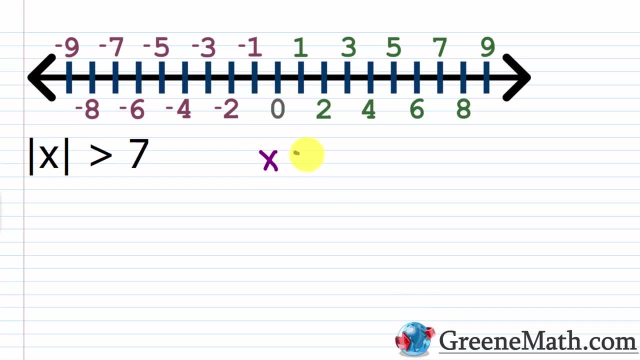 7. we should know that. again, this sets up as x is greater than 7 or x is less than negative 7.. Graphically it's really easy to figure this out. again, I'm thinking about what values here for x have a distance from 0 that is greater than 7.. Well, if I start at, 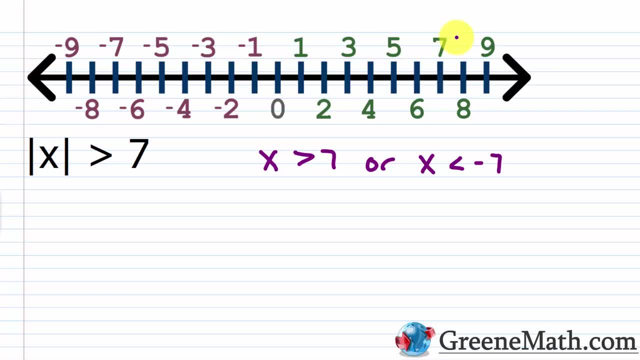 0 and I go 7 units to the right. it can't be 7 itself, but it can be anything larger, right? So I just put a parenthesis at 7 to say it's not included and I shade everything to the right. Same thing goes in the other direction, if I start at 0 and I go 7 units to the left. 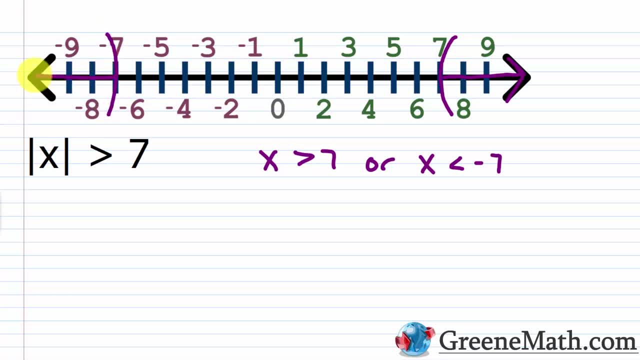 I put a parenthesis at negative 7. I just shade everything to the left like that. So this would be my solution graphically, and we also have this solution here, kind of in our standard notation, and you can even use interval notation if you want. You can say from negative infinity up to, but not including, negative 7, and then the union with 7 is: 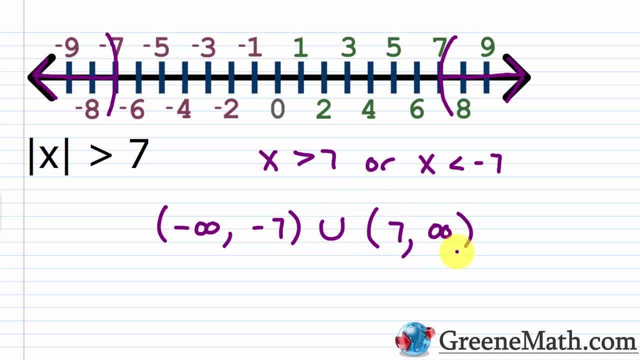 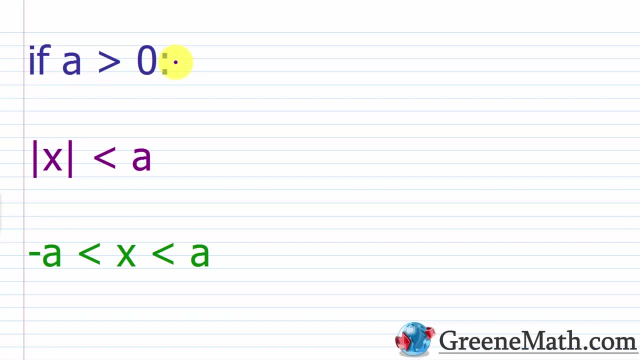 not included again out to positive infinity. okay, So let's take a look at kind of the other scenario that happens. so if a is a positive real number again, if a is greater than 0, if the absolute value of x is less than this positive number a, well then x is going to be between negative a. 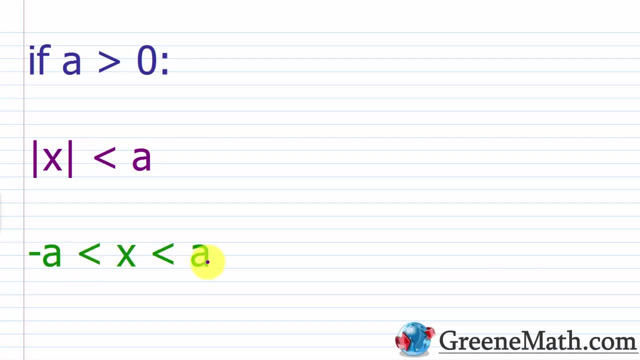 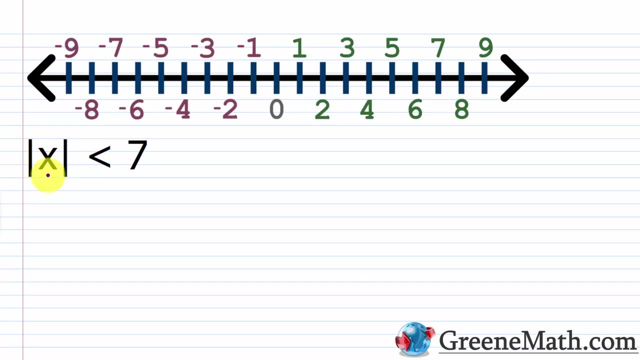 and a right x is greater than negative a and it's less than a. so here we have a compound inequality with and. so let's look at this quick example here. suppose we have the absolute value of x, and now it's less than 7.. So let's look at this quick example here. suppose we have the absolute value of x, and now it's less than 7.. 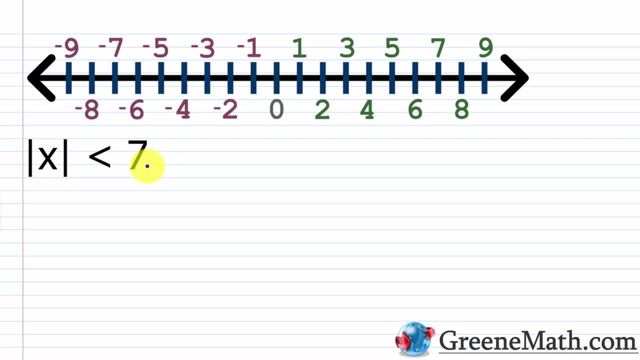 Okay, so we're going to have a compound inequality with, and so, basically, x is going to be greater than the negative of 7 and it's going to be less than 7 itself. Again, basically, to think about this graphically, I'm thinking about all the values whose absolute value or whose distance from 0. 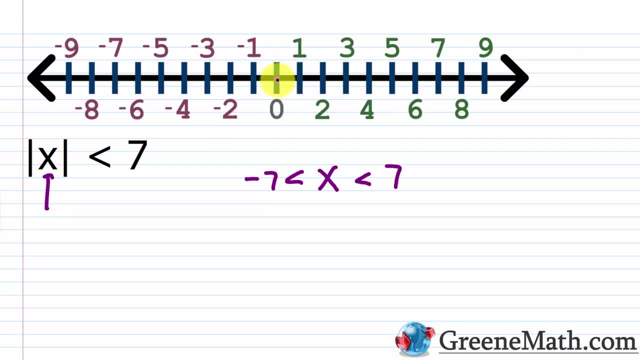 is less than 7.. So, starting at 0, I could basically travel up to, but not including 7. so again at 7- I just put a parenthesis there- and again I could go the direction. so starting at 0, I could go down to- okay, down to- but not include negative 7. so I'd put. 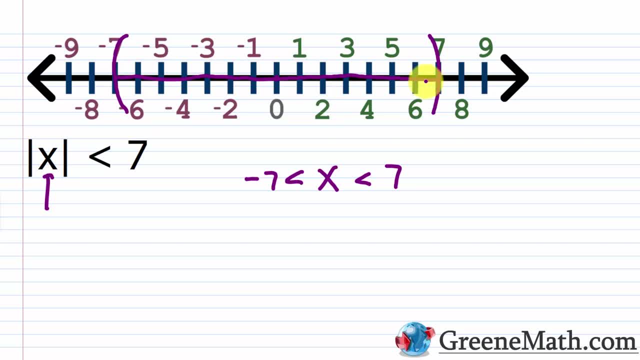 a parenthesis there as well. so that would be my graphical solution: again from negative 7 to 7, with neither of those included, and then in interval notation I'd have negative 7 comma 7, again with a parenthesis next to each. All right, so two special cases that come up that we need to be. 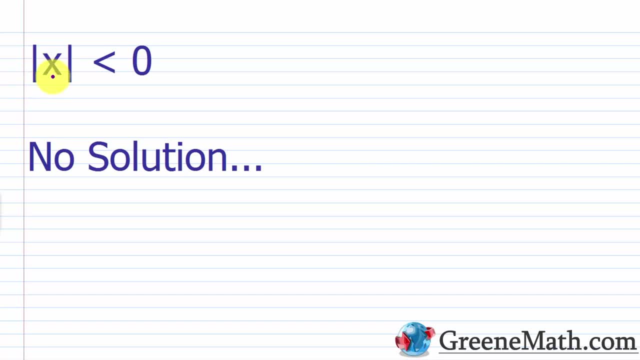 aware of. again, if the absolute value operation in this case is the absolute value of x, if we say a is less than 0, there's no solution here. okay, there's nothing I can plug in for x and take the absolute value of and say that it's going to be less than 0 because the result of this operation 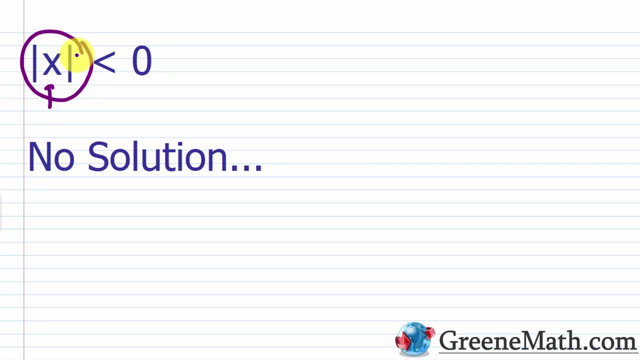 here is going to be 0, which is obviously not less than 0, or it's going to be some positive number, which is also never going to be less than 0. So in this situation there is no solution. and our last special case we're going to come across: if a now is a negative number, if it's less than 0, so some. 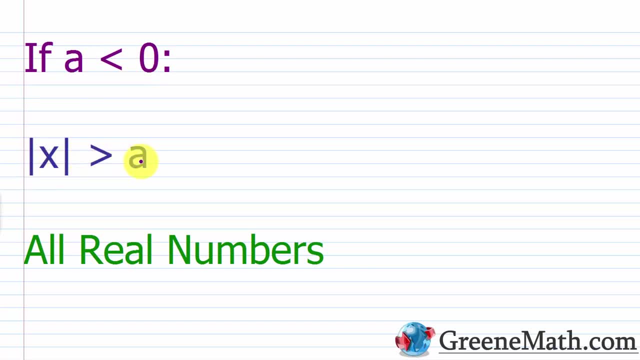 negative real number. The absolute value of x is greater than this negative real number. well then, we're going to have a solution. that's all real numbers, right? if I have, the absolute value of x is greater than negative 5. well, that's always true, right? no matter what I plug in for x, the result of this will: 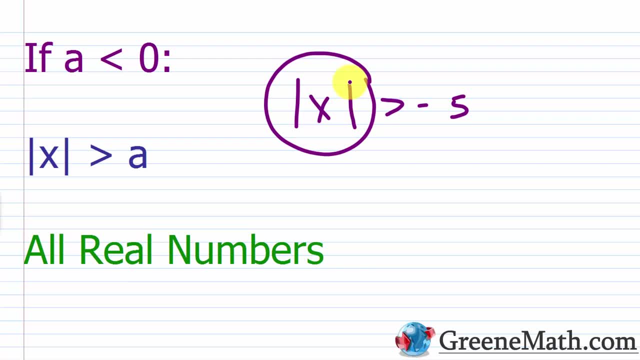 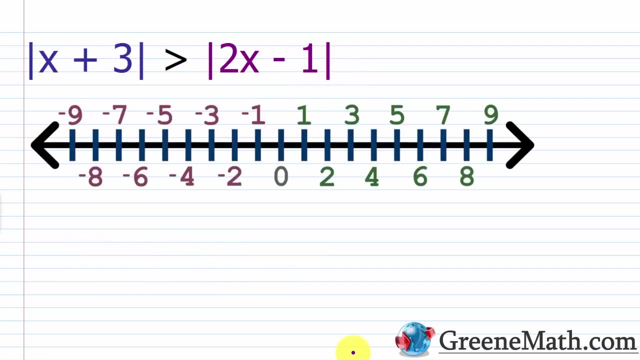 either be 0, which is greater than negative 5, or it'll be positive, which is also greater than negative 5, so this is always true, or you can say true for all real numbers. Okay, so now let's get to the example, and hopefully you saw the lesson where we solved more advanced absolute value. 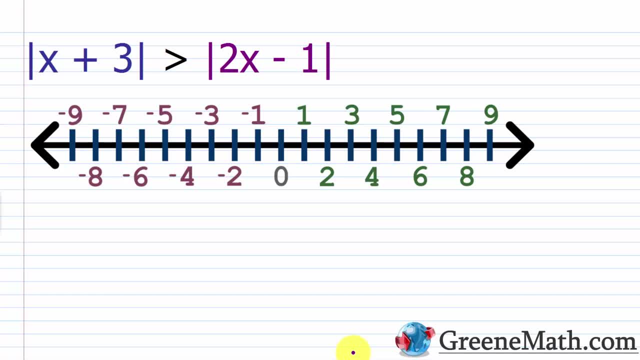 equations. if you did that lesson already, this is going to be a breeze for you. we're basically using the same concepts, okay, so suppose you had something like: the absolute value of x plus 3 is greater than the absolute value of 2x minus 1.. Again, when you look at these, what you want to do, 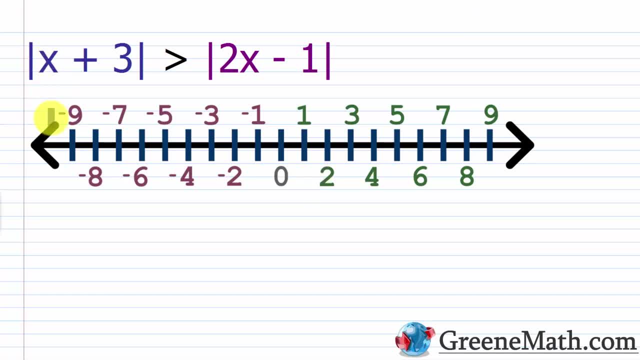 is you want to think about where the expressions inside the absolute value bars are going to be zero. okay, you're thinking about kind of the turning point. so where could this guy go? from positive or from positive to negative? well, that can only happen when that expression is equal to. 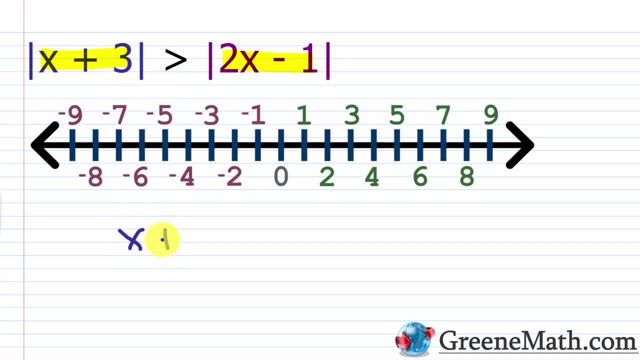 zero, okay. so if I say x plus 3 is equal to 0- and I solve that, I get that x is equal to negative 3, okay. and then, alternatively, if I say that 2x minus 1 is equal to 0, I add 1 to each side of. 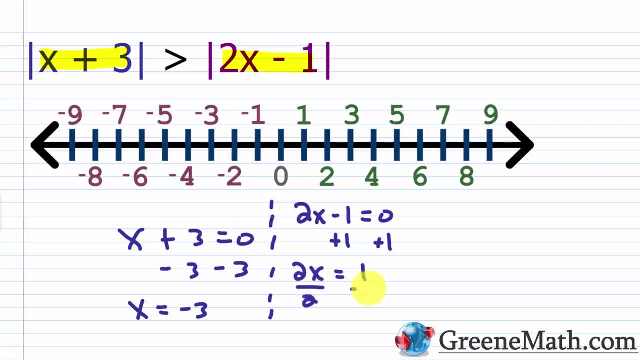 the equation I get: 2x is equal to 1. divide both sides by 2 and I find that x equals 1 half. okay, so I'm going to do this on a table because I find it to be a little bit easier. so the numbers we: 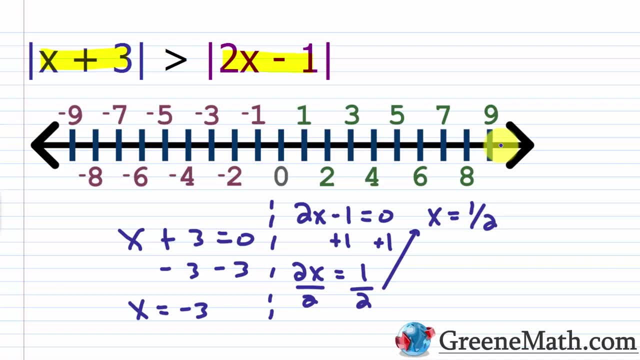 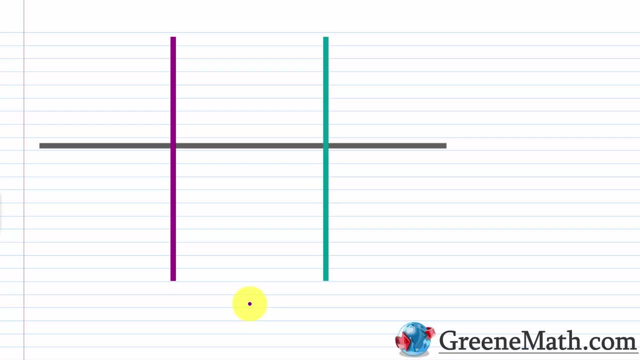 were working with again are negative 3 and positive 1 half, so we're using that to split the number line up into three intervals. I just prefer to do this on a table because it's just easier for me to organize things. so the first interval will be from negative infinity up to, but not including negative. 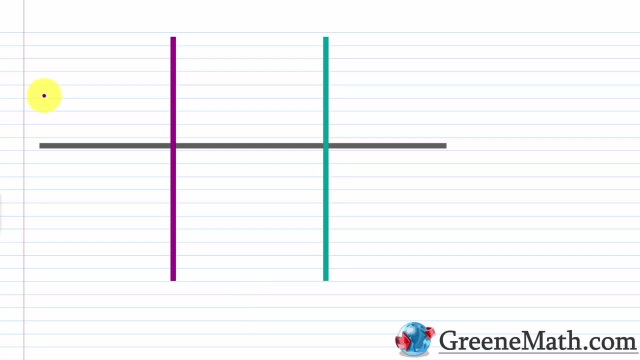 third: okay, so that's my first interval. so I'm going to do this on a table because it's just easier for me to organize things. so the first interval will be from negative infinity up to then my second interval, negative 3. I'm going to include that, okay, and this is going to be out. 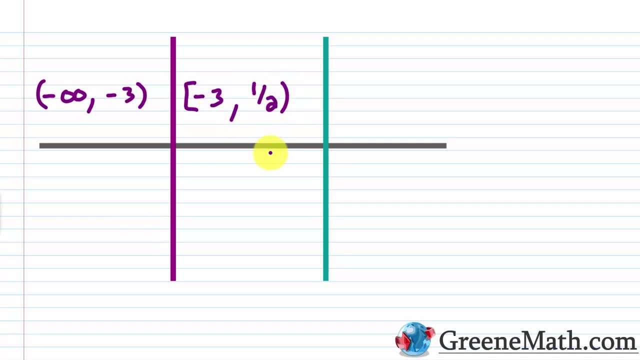 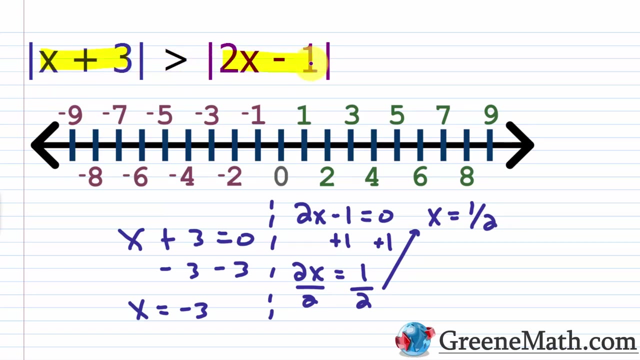 2, but not including 1 half. then my third interval will be anything that includes 1 half or larger. okay, so from 1 half out to positive infinity. now what we're going to do here. let's go back up. so we have: the absolute value of x plus 3 is greater than the absolute value of 2x minus 1. 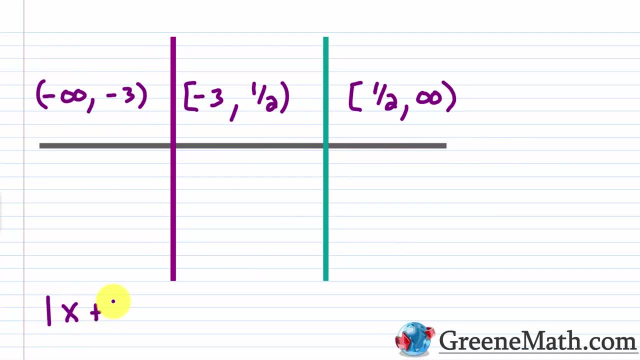 let's go ahead and write that real quick. so the absolute value of x plus 3 is greater than the absolute value of 2x minus 1.. okay, so what we're doing here is we're looking at each interval. we're thinking about is the expression inside the absolute value bars. 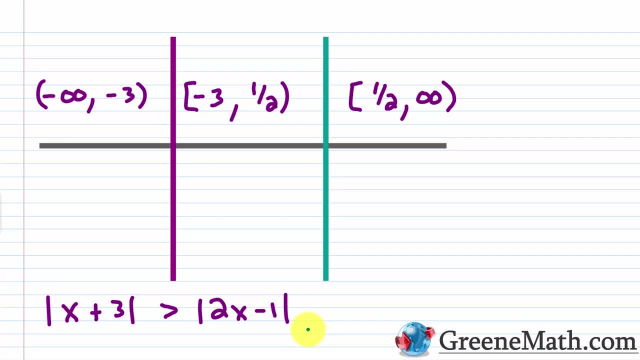 negative, is it zero or is it positive? okay, that's what I want to consider. so, for this guy right here, think about the fact that in this interval it's going to be negative. right, I know that x plus 3 is equal to 0 when x equals negative 3.. so anything less than negative 3. 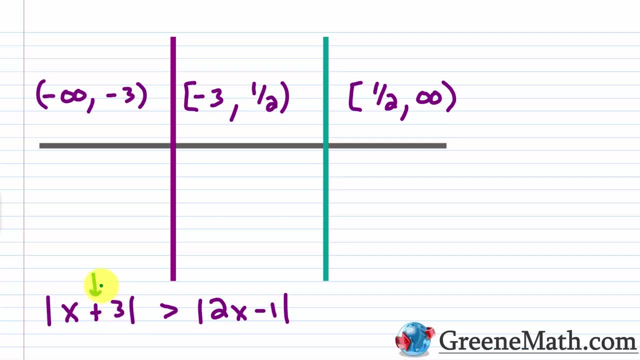 means it's going to be negative, right? so in this interval I will replace this expression here, this absolute value of x plus 3, with the negative of x plus 3.. so I just wrap it in parentheses and put a negative out in front to express that. okay for this guy, right. 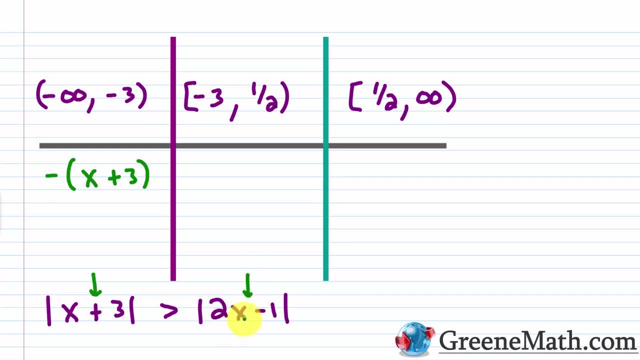 here, this 2x minus 1, it's also going to be negative, right? because 2x minus 1 is going to be zero when x is one-half. so if we're less than a half, which we are in this case, it's going to be. 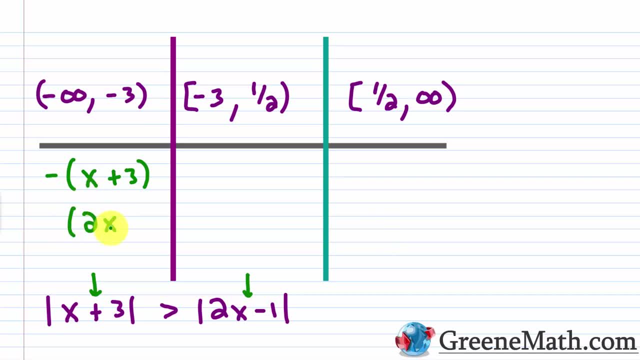 be negative. so again, I just wrap it in parentheses. so 2x minus 1, put a negative out in front. okay, and we'll deal with this scenario in a second. let's just kind of move on and write everything. so in this interval here we have from negative 3 up to, but not including one half. so at negative 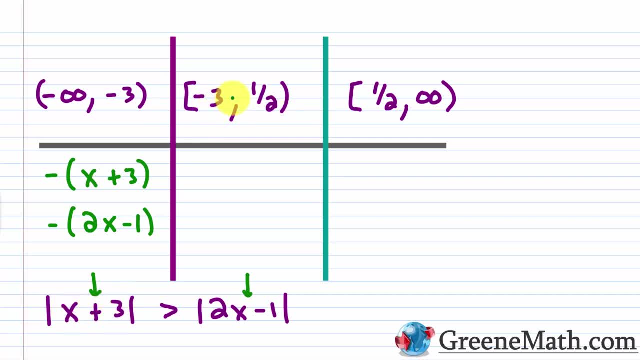 3. we know that this guy would be 0, but anything larger than that means it's going to be positive, okay. so whether it's 0 or some positive value, I can just take the expression itself. so I can just say it's x plus 3. here and again, this is still in a format of where it's larger than negative 3. 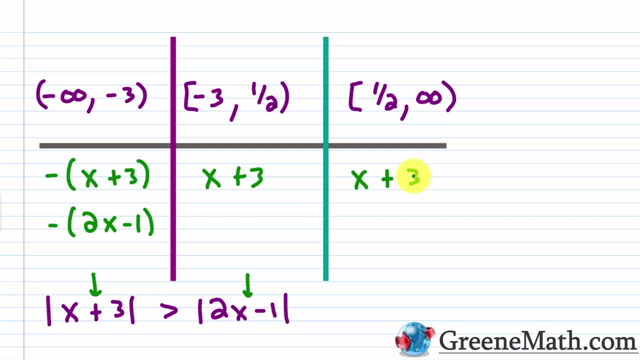 so in this interval it'll also be just x plus 3. okay, then, for 2x minus 1, again, it's made 0 when x is one half, and this interval between negative 3, including negative 3 up to but not including one half, it's still going to be negative, right, because that's less than one half. so I would say: 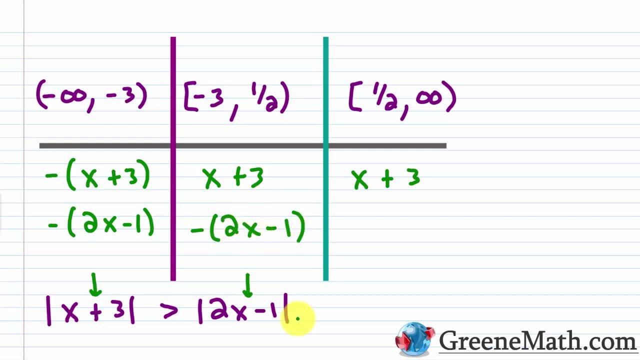 the negative of 2x minus 1, and then here it could either be 0, if x is a half, or some positive value. So I just drop the absolute value bars and write the expression: So two X minus one. Okay, So a very simple process. Again, if it's zero or positive, 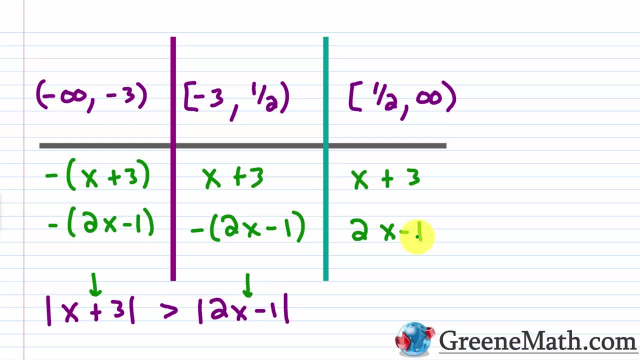 in that interval, you replace the absolute value expression with just what's inside the absolute value bars. Okay, That's all you need. If it's a negative, okay, then what you want to do is drop those absolute value bars, wrap it in parentheses, put a negative out in front. You're basically. 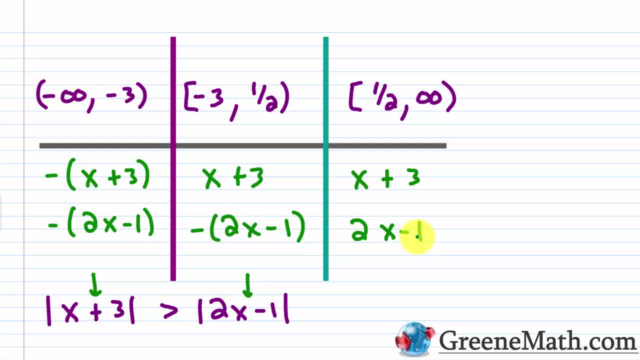 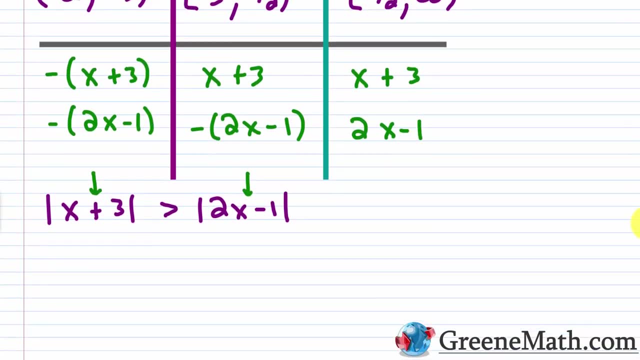 changing it into its opposite. All right, So now we've got a lot of work to do. We've got to go through the different possibilities. So the first possibility is that both of these are negative. So let's kind of scroll down and crank that out. So I'm going to have the negative of X plus three. 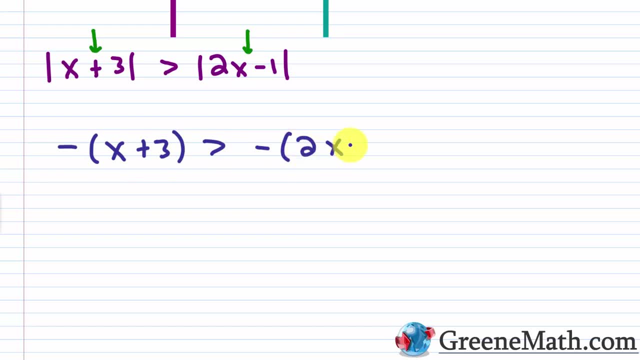 is greater than the negative of two X minus one. Now, if we want, we can clear the negatives by just dividing both sides by negative one. But again, because we're working with inequality and we divide it by a negative, we've got a flip. 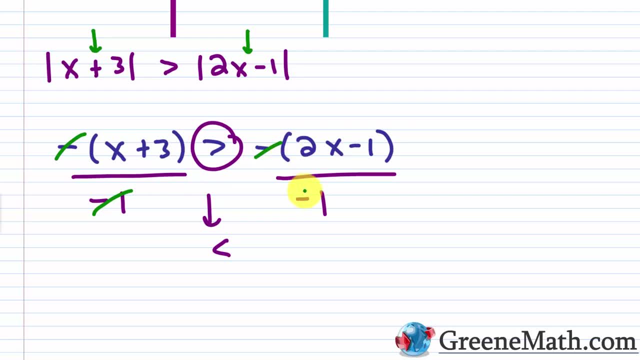 Okay, So this is going to cancel and this is going to cancel. You have X plus three. now is less than two. X minus one. Let's go ahead and subtract two X away from each side of the inequality, And let's also subtract three away from each side of the inequality. So this is: 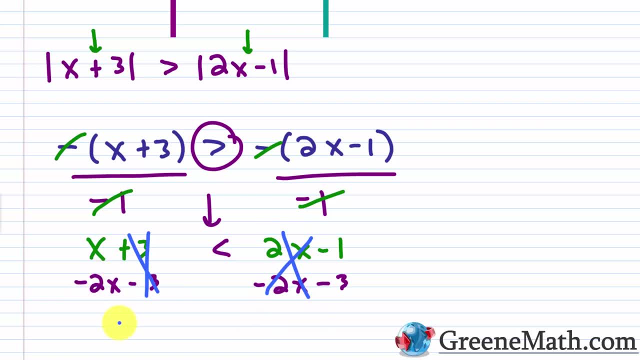 going to cancel. This is going to cancel. We'll have X minus two, X, which is negative, X, And this is less than you've got negative one minus three, which is negative four. As a final step, let's divide both sides by negative. 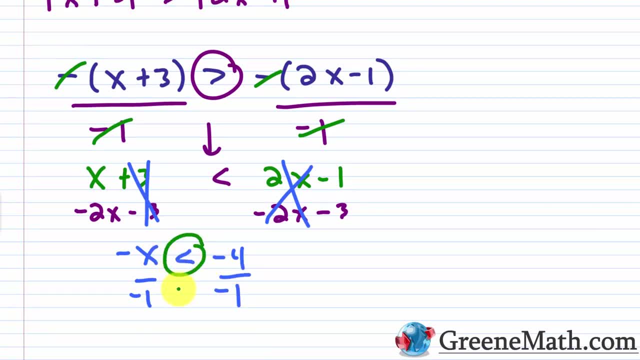 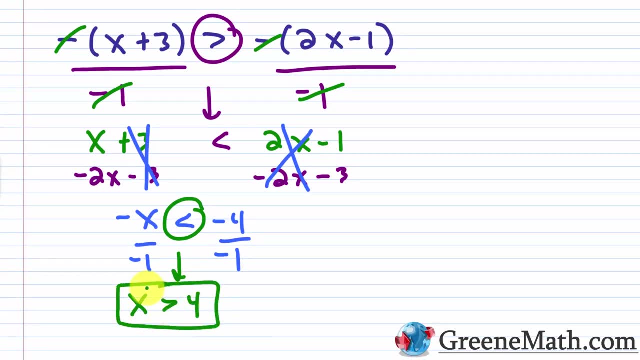 One And again we divided by a negative. So flip this guy, You're going to get that X is greater than four. Okay, So X is greater than four. Now we want to compare X is greater than four to the interval that we're working with. The interval that we're working with specifically says that: 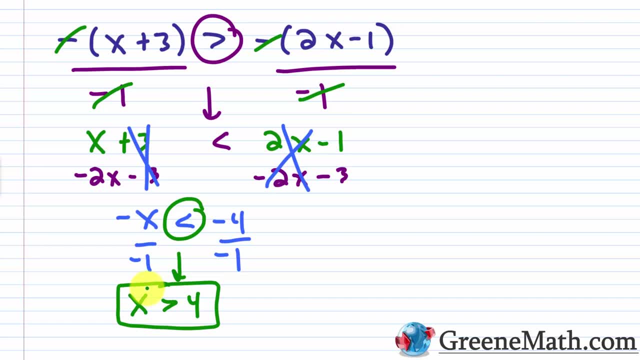 X is basically coming from negative infinity up to, but not including, negative three. X is greater than four is not in that interval. So this solution is going to be rejected. Okay, Let me erase all this. So I'm going to kind of write it in the column. So I'm just going to write: X is greater than four. 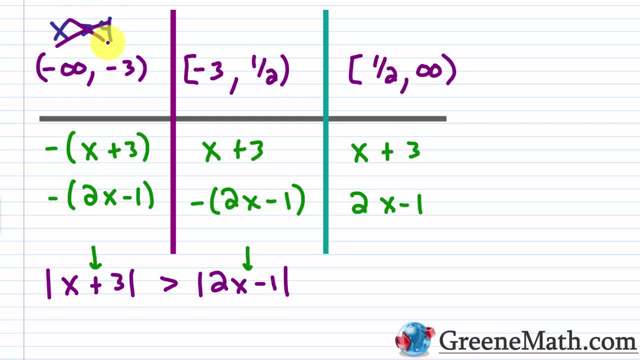 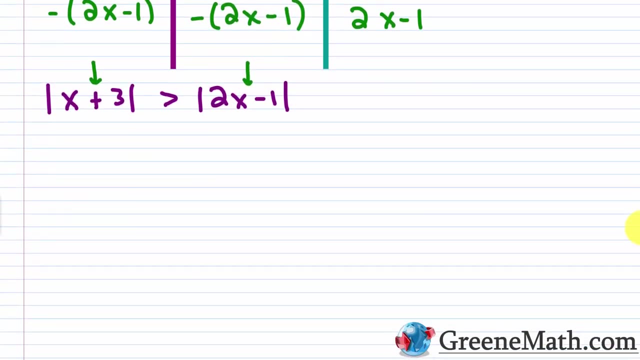 here And again, this is not within our interval, So we reject that solution. Okay, Now let's think about this interval here again, where the X plus three is positive and we're going to use the negative of two X minus one. Okay, So let's scroll down and we're going to say that we have X plus. 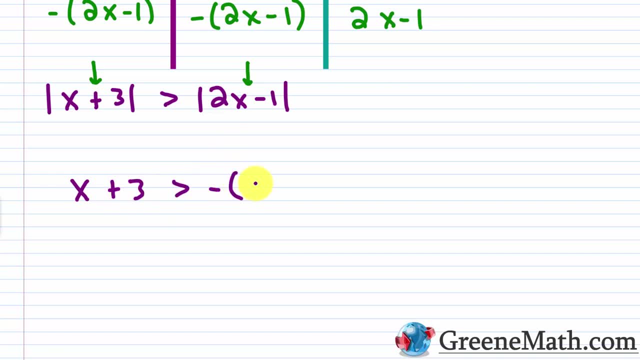 three is positive, And then this guy is going to be negative. So the negative of two X minus one. Okay, So I'm going to go ahead and solve this guy. I'm going to distribute this. This will be negative: two X plus one. So if I add two X to both sides of the inequality and I subtract three away from, 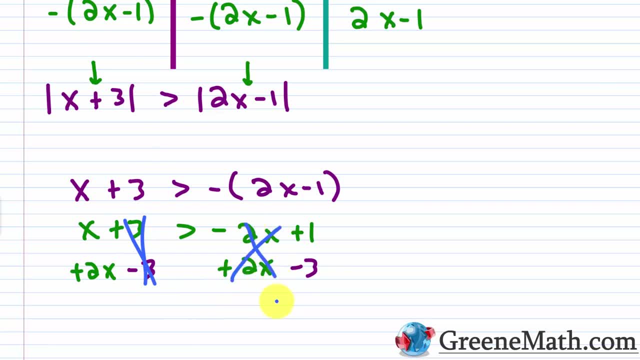 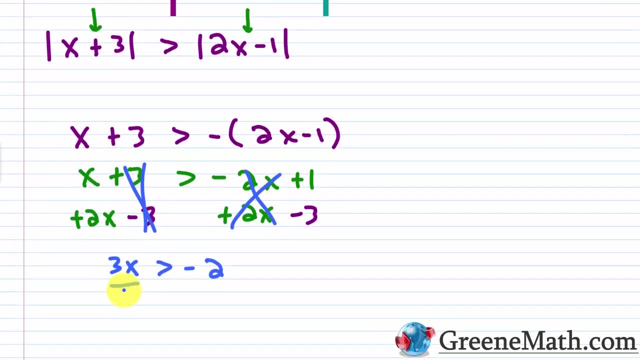 each side of the inequality. this will cancel. This will cancel. X plus two. X is three. X- This is greater than one minus three is negative two. Divide both sides by three And we get that X is greater than negative two thirds. Okay, So let me erase this real fast. 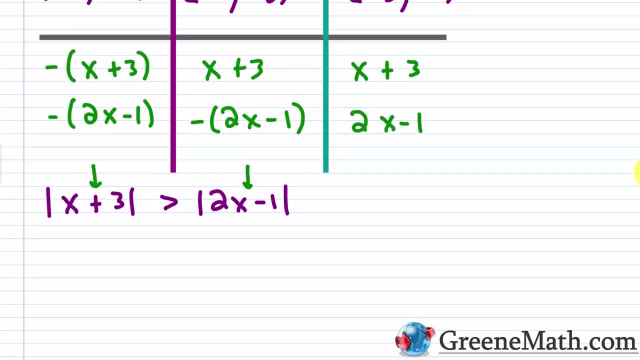 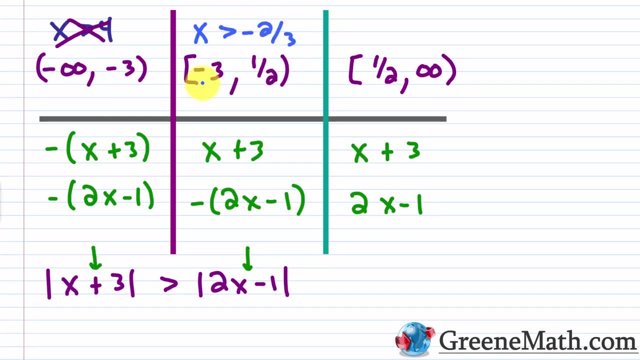 X is greater than negative two thirds. Let me write that up here. So X is greater than negative two thirds. Okay, Is that? in our interval, The interval is from negative three, including negative three, up to, but not including one half. Well, yeah, it is. So this is a partial solution. 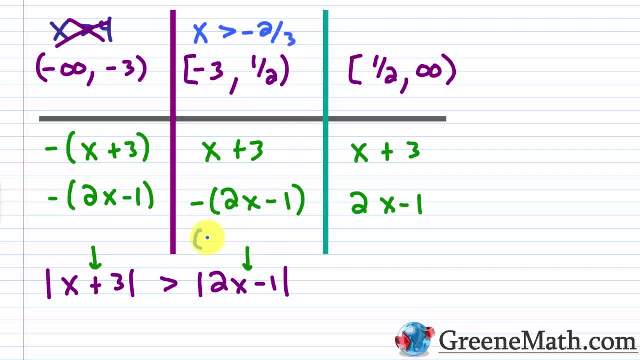 Okay, So for right now I'm just going to write this guy as, again, not including negative two thirds, because it's strictly greater than up to, but not including one half. Okay, And then we'll think about this solution And if we have a solution there, 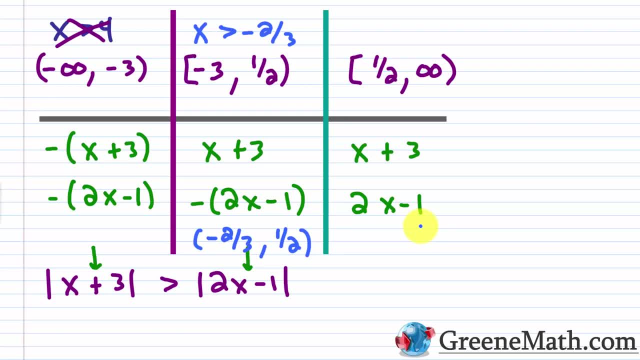 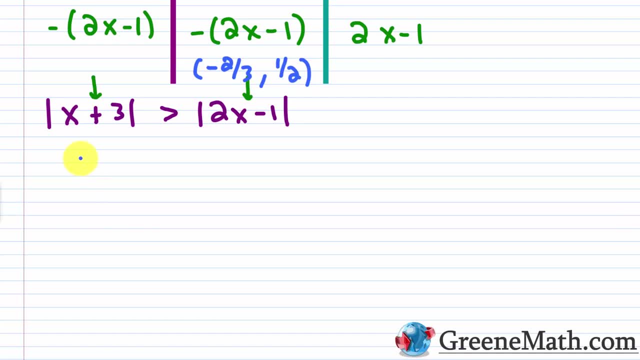 we'll have two partial solutions we can put together as a full solution. Okay, So in this case everything's positive, So we can just drop the absolute value bars and go with what we have. So you'd have: X plus three is greater than two. X minus one. Let's subtract three away from each. 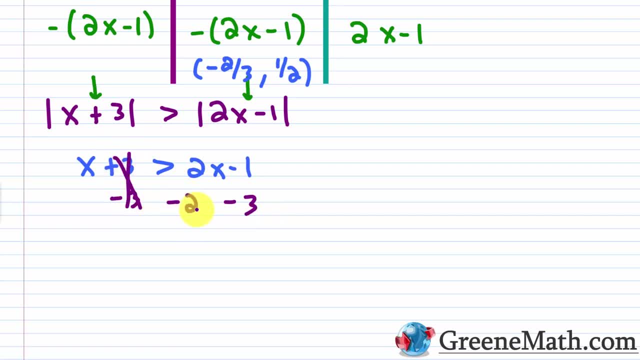 side of the inequality, So that would cancel. Let me subtract two X away from each side of inequality, So that would cancel. X minus two. X is going to give me negative X. This is greater than negative One minus three is negative four. Let's divide both sides by negative one, So we know that this. 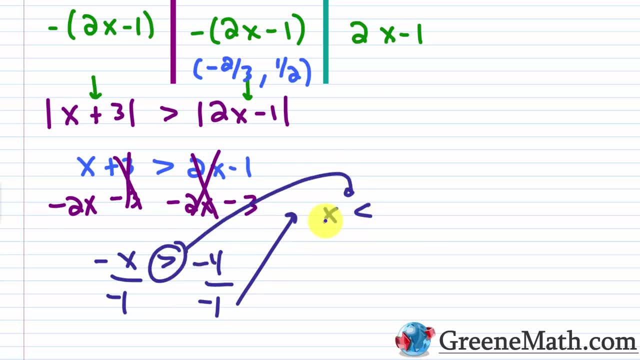 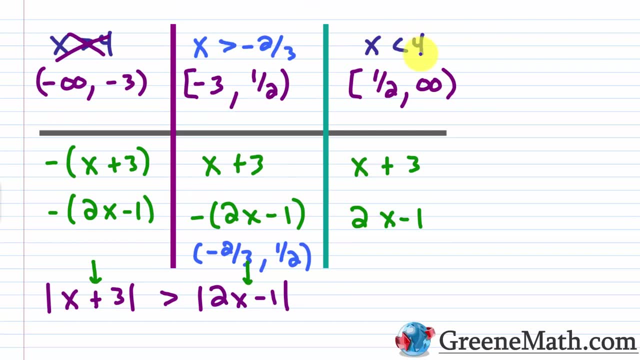 is going to flip right, So this is going to end up being a less than. So you have, X is less than positive four. Okay, So again, let me erase all this. So we say X is less than four, Does that? 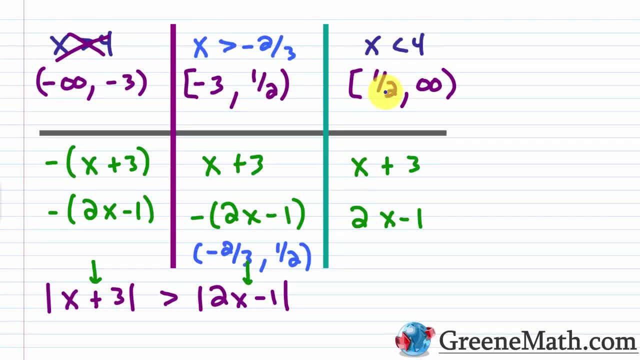 fit in our interval. Yeah, it does Right, Because we have from one half, including one half, out to positive infinity. X is less than four fits in there. You could basically say it's another partial solution. You would include one half and you're. 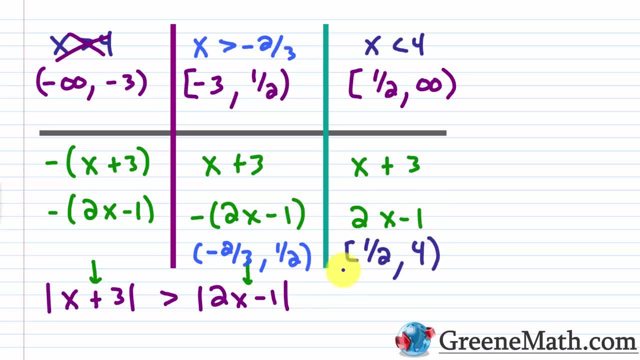 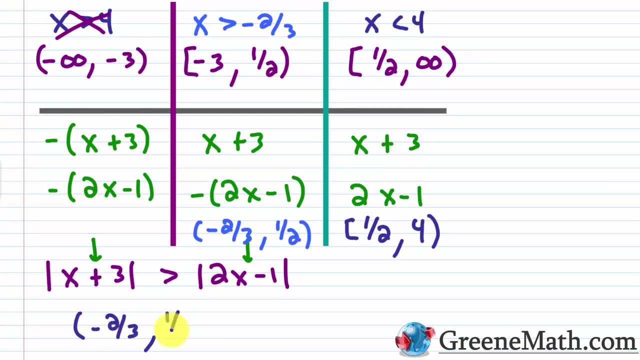 going to go up to but not include four. Okay, So if I take these two partial solutions- and I just take the union of the two, So again from negative two thirds, not including that, up to but not including one half, and the union with you have one half which is included up to four. Okay, So this: 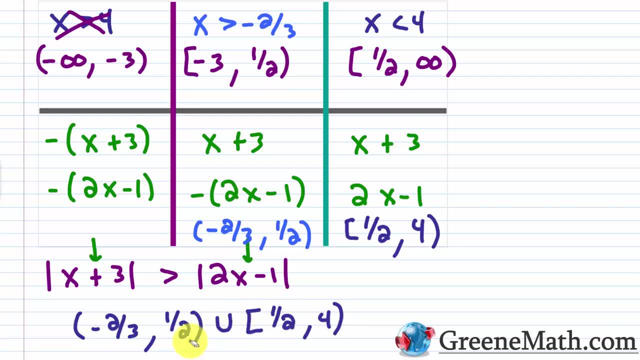 would be your solution set And basically, when you combine the two, you can get rid of this part right here and just kind of slide this down, And that's what you're going to get. right. You're going to get from negative two thirds, not including one half. So this would be your solution set And 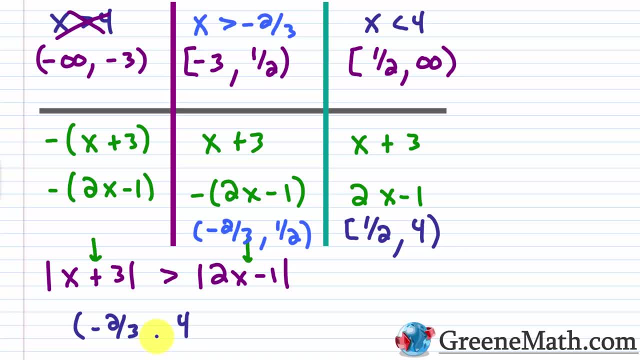 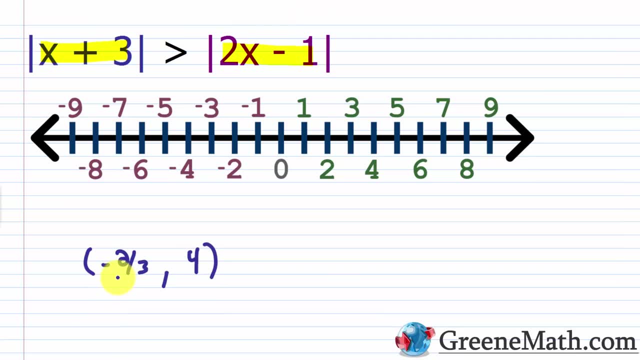 again, from negative two thirds, not including that up to, but not including four. Okay, So let me kind of drag this up to our original page and we'll paste our solution here again: from negative two thirds, not including that up to and not including four. So negative two thirds, let's. 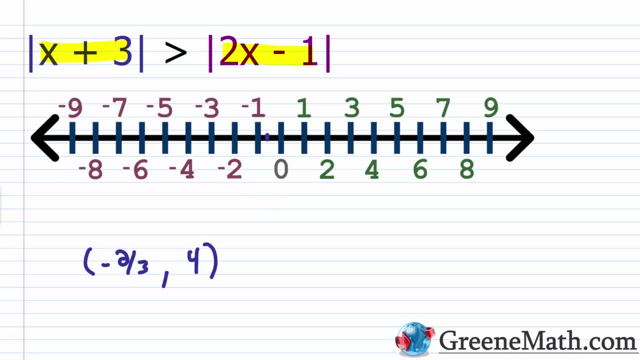 just go ahead and say: that's about right here, And I'm just going to mark that and say: this is negative two thirds. So I'd put a parenthesis there because it's not included. Four is not included. Just shade everything in between, Okay, And then we can go ahead and say: this is 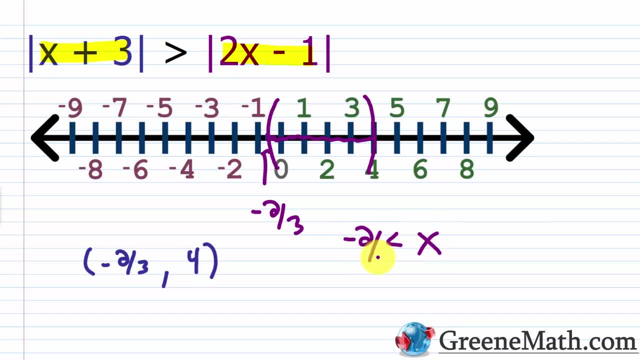 negative two thirds, Okay. And then we can also write this saying that X is greater than negative two thirds and less than four: Okay. So this is your interval notation, This is your standard notation, And then this is graphically. So those are the solutions for, again, the absolute value. 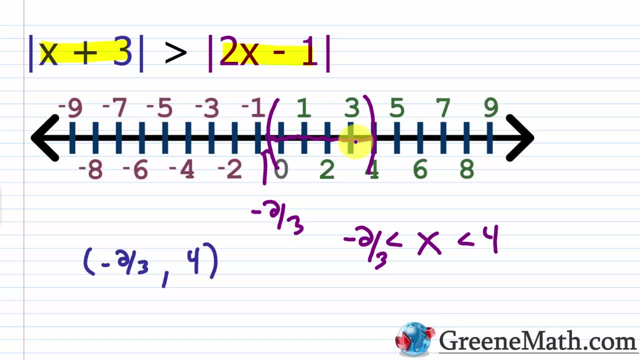 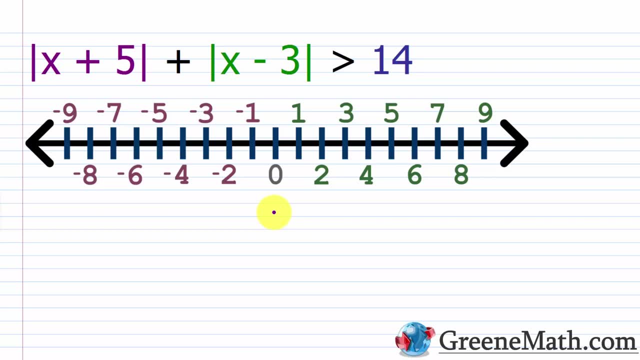 of X plus three is greater than the absolute value of two X minus one. All right, let's go ahead and take a look at another example. So this guy here is going to be a little bit more complicated, but we're going to solve it using the same strategy. So we have the absolute value. 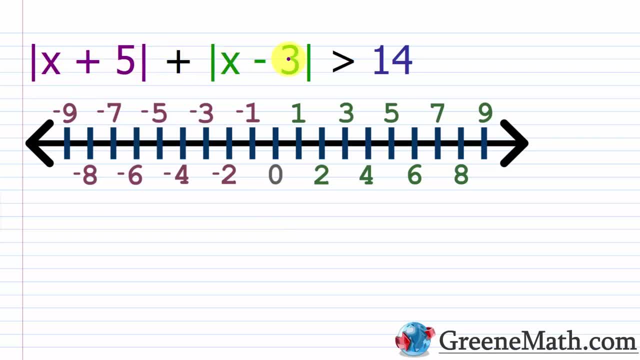 of X plus five, And then plus, we have the absolute value of X plus five, And then plus, we have the absolute value of X minus three, And then this is greater than 14.. So the first thing we want to do is just take what's inside of the absolute value bars in each case. So this expression here: X plus. 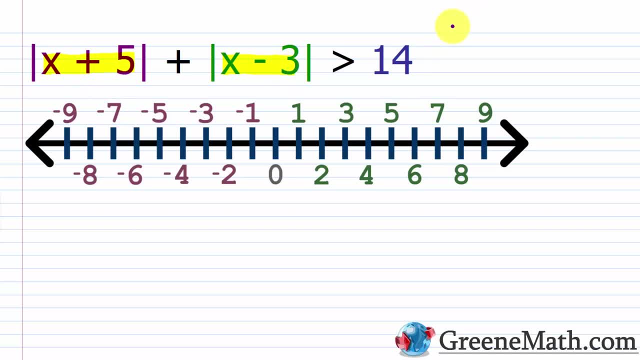 five and this expression here, X minus three. we just want to set those guys equal to zero and see what the result is. So if we have X plus five equals zero. very simple: subtract five away from each side of the equation we get X is equal to negative five. Then for the other guy we have 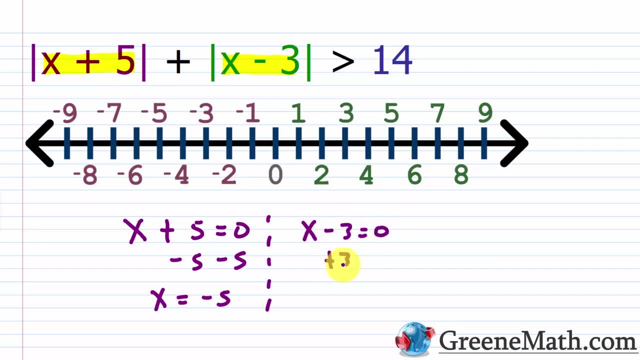 X minus three. So X minus three, we get X plus five. And then we have X minus three. we get X equals zero. Add three to both sides of the equation, we get X is equal to three. So again, these two numbers are going to help me split the number, line up into kind of three intervals. 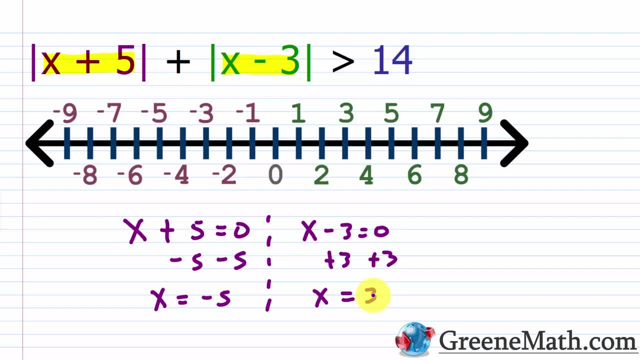 We're going to have from negative infinity to negative five, with negative five not being included. Then we'll have negative five to three, with negative five included and three not, And then three included in anything larger. Okay, so let's set this up using a table Again. 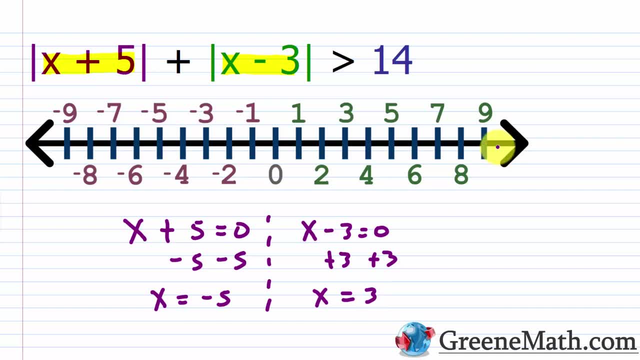 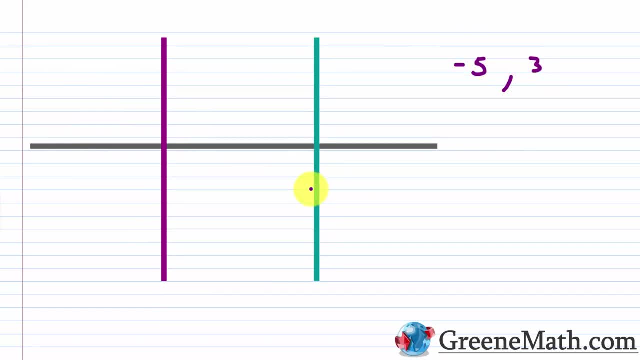 I don't like to use the number line itself. I like a little table. It helps me organize things. So again our numbers. I'm just going to write them here. We have negative five and positive three. So again, from negative infinity up to, but not including, negative five. 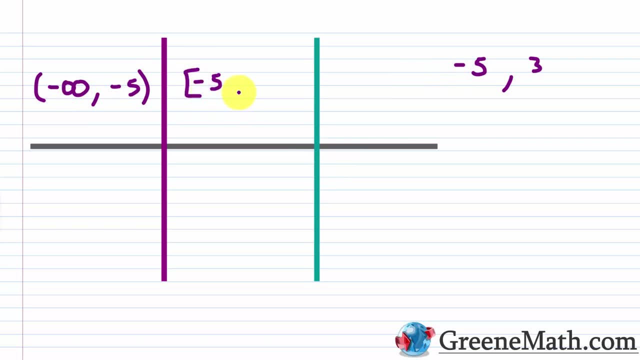 And then negative five will be included here. So negative five is included And then up to, but not including, three, And then three will be included and then out to positive infinity. Okay, so let's rewrite our inequality Again. if we go back up, we have the absolute value of X plus five. 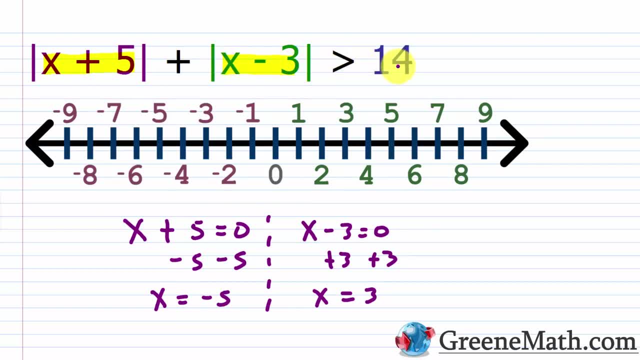 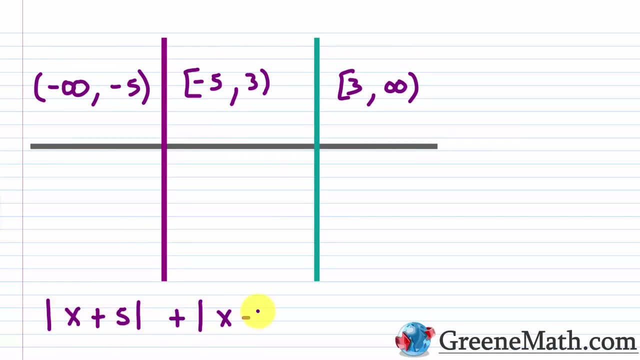 then plus the absolute value of X minus three, And this is greater than 14.. So let's write that: So we have the absolute value of X plus five, And then plus, we have the absolute value of X minus three, And this is greater than 14.. Okay, so we know in this. first, 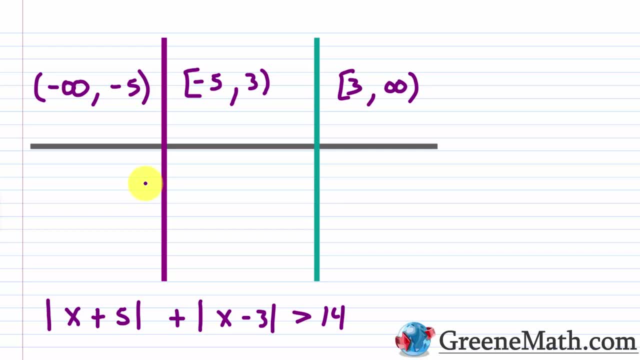 interval, the one all the way to the left where we're coming from- negative infinity going up to, but not including negative five. Both of these guys are going to be negative, right? This guy right here is going to be negative because it's zero, or X equals negative five, right? So we're. 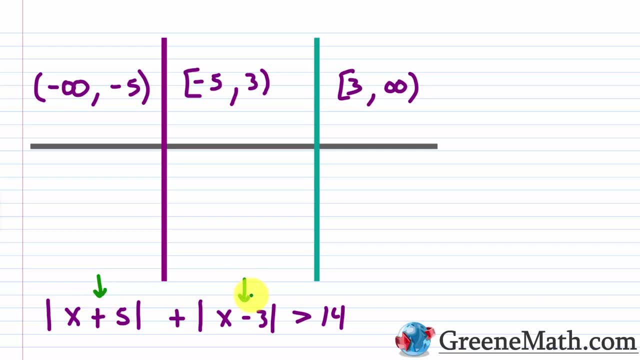 less than negative five. So this guy's negative. This guy is also negative because it's zero when x equals three, and we're definitely less than three in this case. So we're going to say that this guy is the negative of x plus five, And this guy is 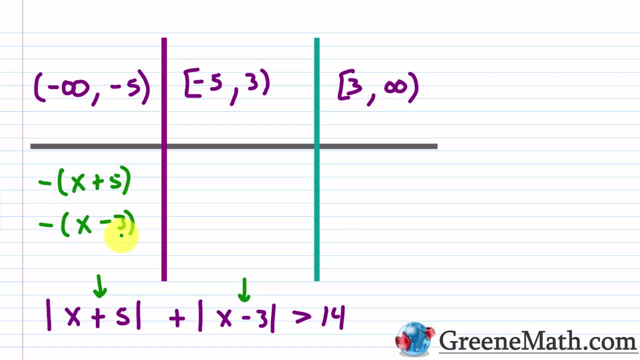 going to be the negative of x minus three, Okay, And then, in this case, right here, now, we're from negative five, including that, up to three, but not including that. Well, now, this guy right here, this x plus five, that expression is going to be either zero or positive. 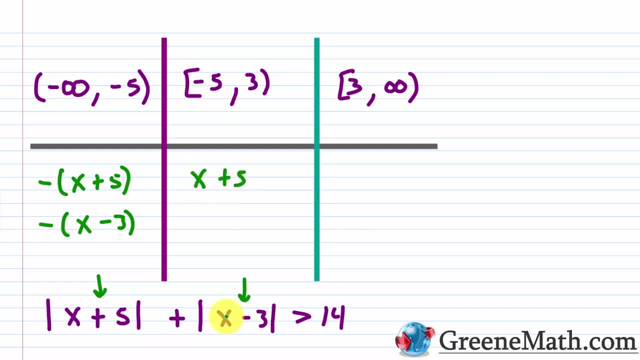 So we're going to replace it with the expression itself. So we'll put just x plus five. And then this guy right here, this x minus three is still going to be negative, right? Because again it's zero. when x is three, we're less than three, So it's still gonna be negative. So we put the negative. 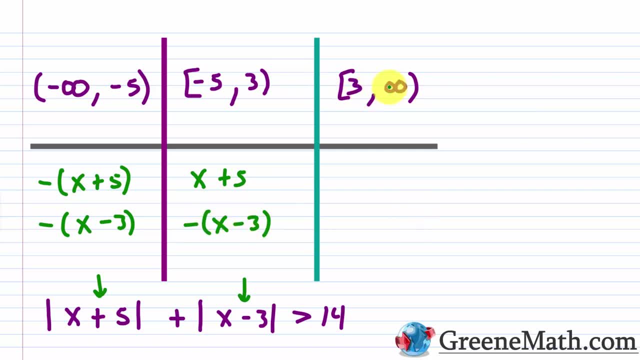 of x minus three. And then this last case where we're three or anything larger. well then this x plus five is going to be positive. And then for x minus three, that could be zero or positive. So again, we just put x minus three there, Okay? So again, if it's zero or positive, you just take. 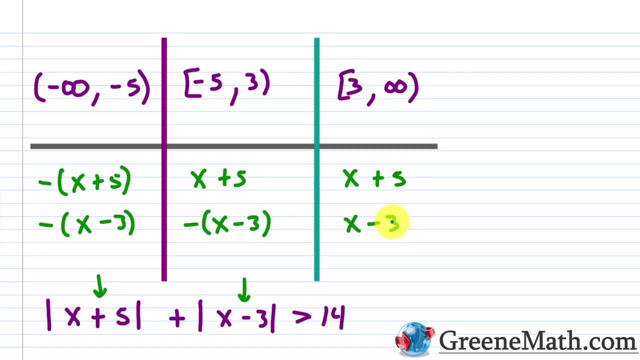 the absolute value bars and you can write that down, basically thinking about: just drop the absolute value bars If it's negative, well then you drop the absolute value bars, wrap it in parentheses and then put a negative out in front. Okay, So that's all we're doing, All right? So? 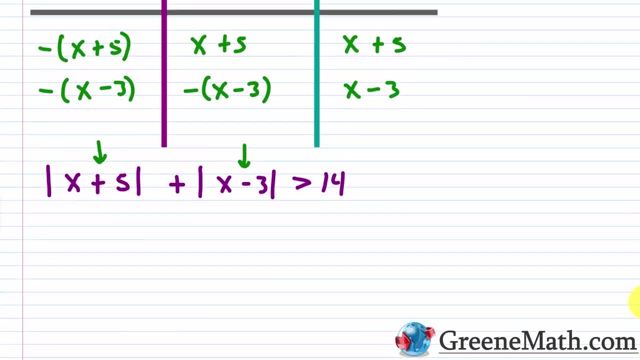 let's go through the possibilities now Again. this is the tedious part. So in the first case both are negative. So I have the negative of x plus five, then plus the negative of x minus three, And you can just put the minus there instead of plus negative. doesn't really matter. 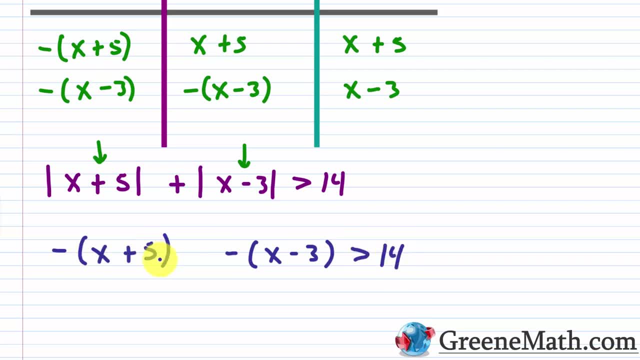 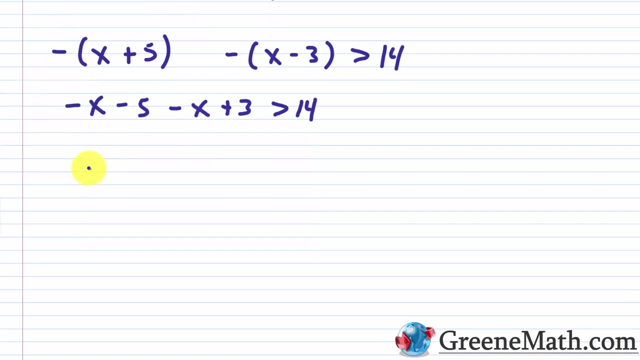 And greater than 14.. Okay, So I'm going to distribute this negative to each term. I'm going to have negative x minus five, and then minus x plus three, and this is greater than 14.. Let me scroll down and get a little room going. So I know that minus x minus another x is negative. 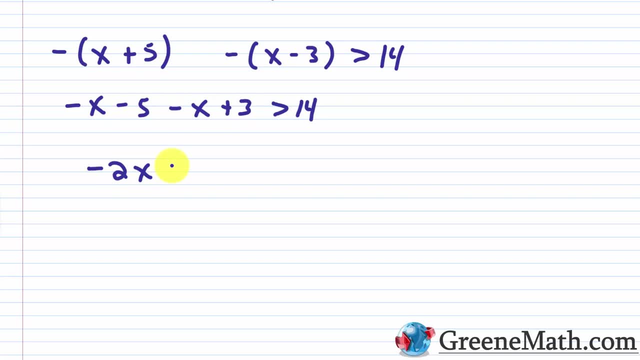 two x. I know that minus five plus three is negative two. this is greater than 14.. Let me go ahead and add two to both sides of the inequality. we know this will cancel. Negative two x is greater than 16.. So then, when I divide both sides by negative two- remember we got to flip- 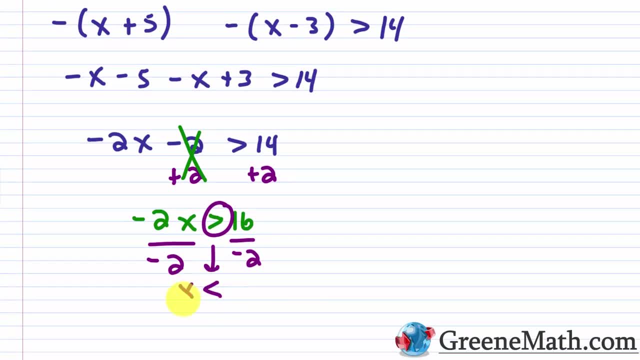 this, So this becomes a less than now you'll have x is less than negative eight. Okay, so x is less than negative eight. Is that in the interval that we're working in right now? Well, yeah, we said that our current interval is anything less than negative. five negative eight is definitely less. 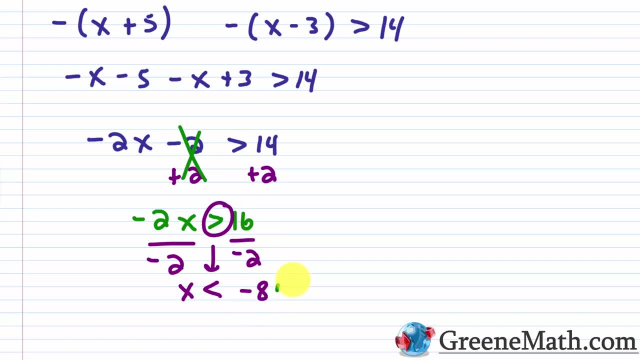 than negative five. So we're good to go right. This is going to be a valid solution for us. But again, it's just part of our solution, because we might have to do something else, So we're going to have more to come. Okay, so we just consider it as a partial solution for now. Alright, so let me 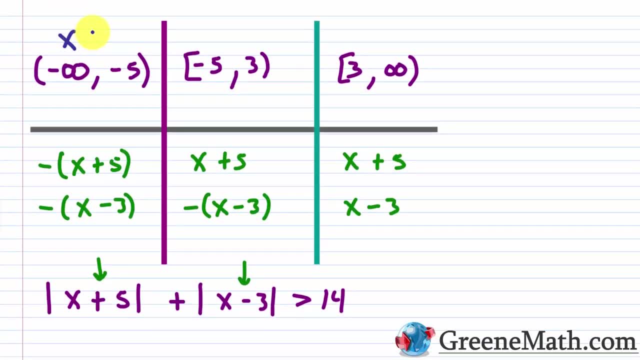 erase all this. So again, for this part, I said that x was less than negative eight And I'm gonna go ahead and just put a checkmark there. So we know that we accepted that solution. Alright, for the next interval, again from negative five and including that, up to, but not including three. 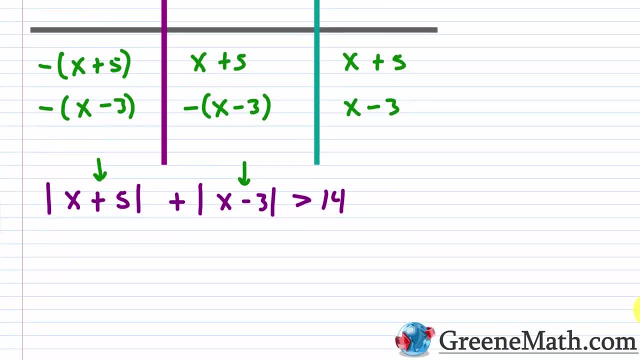 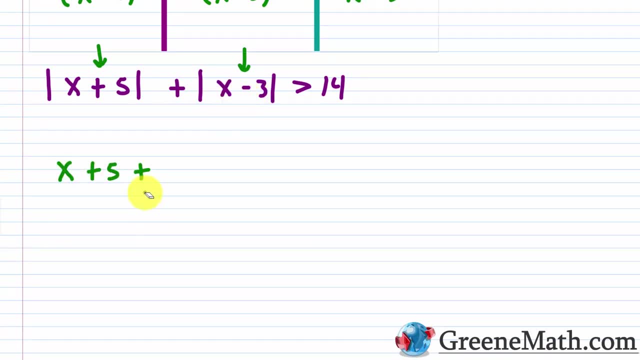 this guy's positive, this guy's negative. So let's go ahead and do that. So x plus five, again that's positive. and then plus this x minus three, that expression is gonna be negative. So I'm gonna put minus the quantity, x minus three, And before we continue, let's just go. 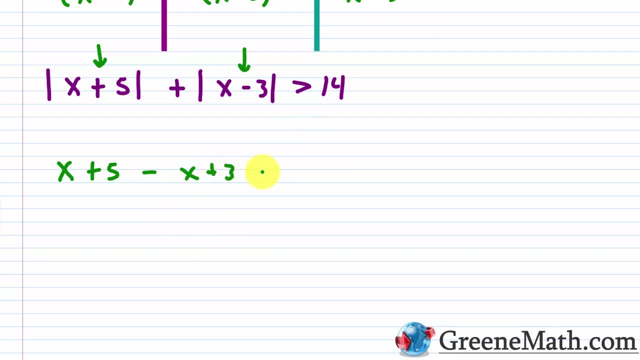 ahead and distribute this, So this would be minus x and plus three. make that a little quicker. then this is greater than 14.. Okay, so x minus x, that's going to drop out. So this is gone, right. So you basically have that eight is greater than 14, which is false. okay, that's never going. 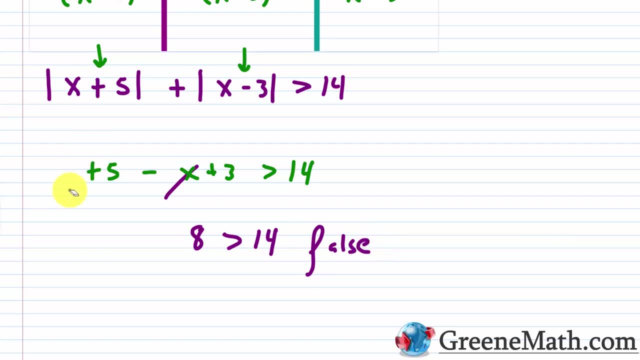 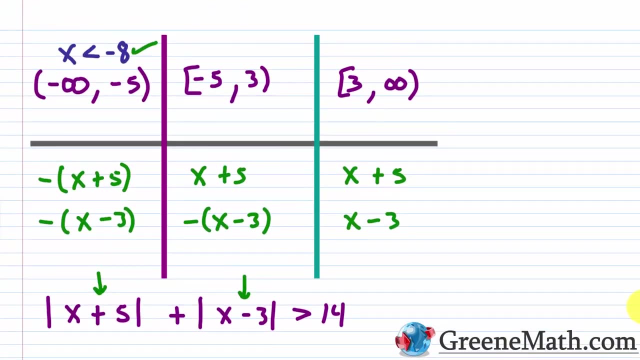 to be true. So nothing's going to work in that interval. So you don't even have to put anything, you just say it doesn't work. Alright, so the next one we're going to look at: we have from three and including three out to positive infinity, And again both expressions. 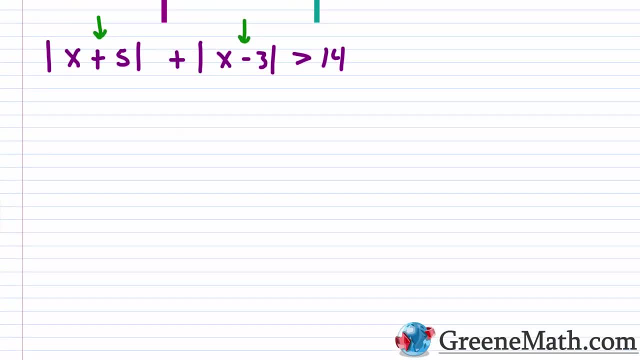 are positive here, So we can just drop the absolute value bars in this case. So we just say x plus five plus x minus three is greater than 14.. So x plus x is two x, and then five minus three is two, so plus two, and this is greater than 14.. Alright, so let's subtract two away from each side. 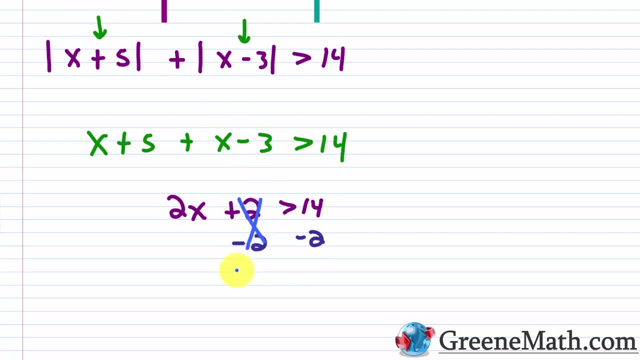 of the inequality, And then we can cancel this. we'll have two: x is greater than 14.. And then we'll have two x is greater than 12.. Let's divide both sides of inequality by two. we'll find that x is. 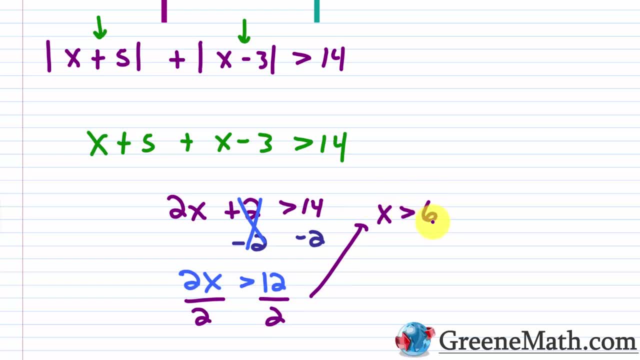 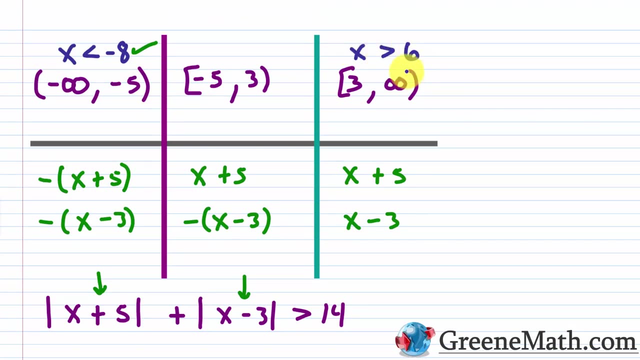 greater than six. okay, x is greater than six. is that in our interval? Well, yeah, this interval is from three out to positive infinity. x is greater than six. that is in the interval. So we're basically good to go with that. So let's erase this. we'll say x is greater than six. Let me put 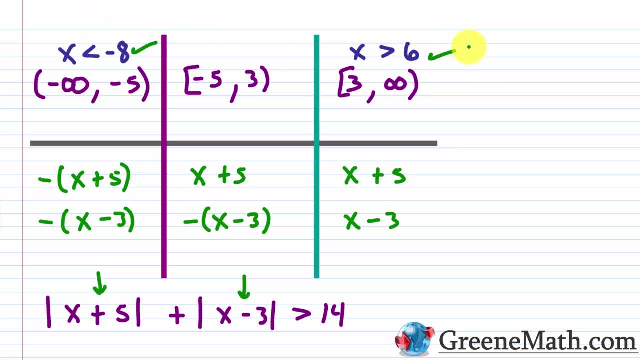 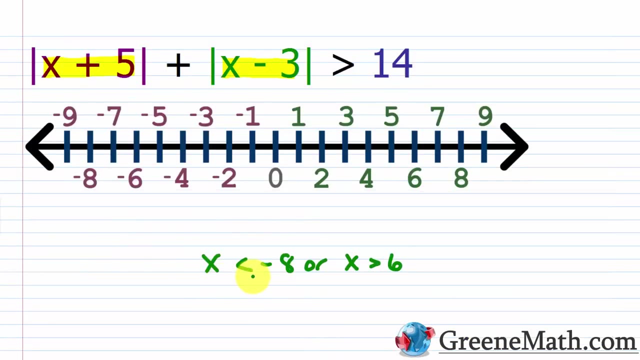 a checkmark there. So basically we would just combine these two As one statement. we would say: x is less than negative eight or x is greater than six. So let me just copy this real quick, Go back up And let me just paste this in. So again, x is less than negative eight. So find 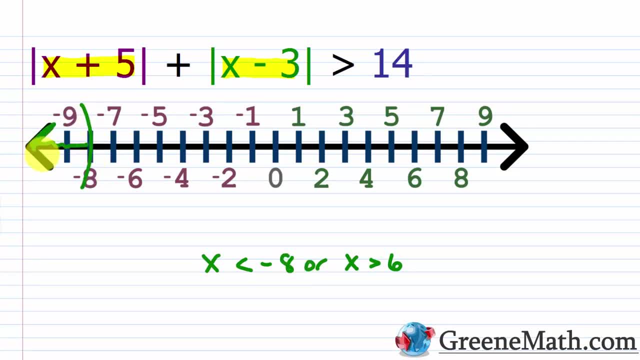 negative eight. I'm going to put a parenthesis there, I'm just going to shade everything to the left. Or also, x could be greater than six. So find six, put a parenthesis there, shade everything to the right. Okay, In interval notation again, I could just say from negative infinity. 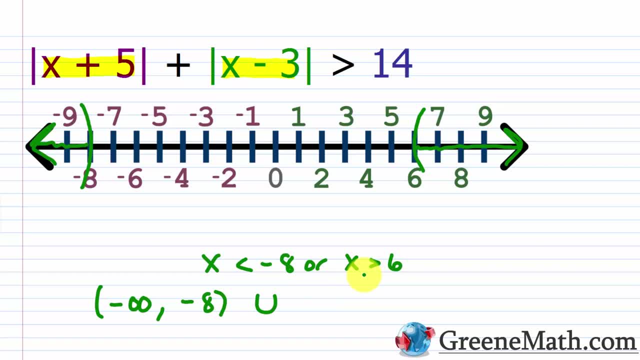 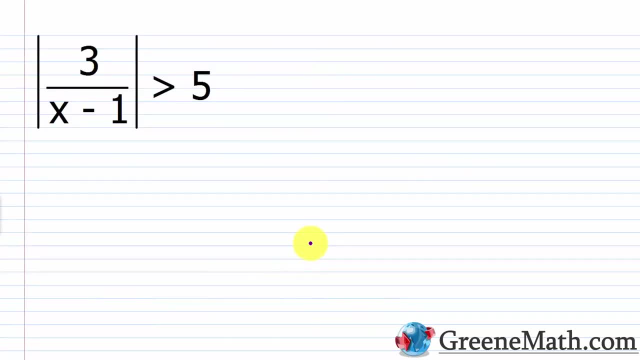 up to, but not including negative, eight and the union with anything larger than six, right, So in both cases I'm using a parenthesis to show that it's not included. All right, so let's kind of change things up and look at another common type of problem that you'll see in this section. 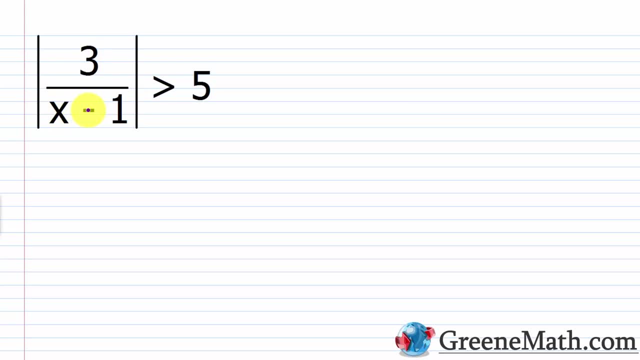 So let's suppose we saw something like the absolute value of three over x minus one, and this is greater than five. So how can we solve this type of problem? Well, one approach is to have this absolute value operation. First and foremost, there's one of them, and it's already. 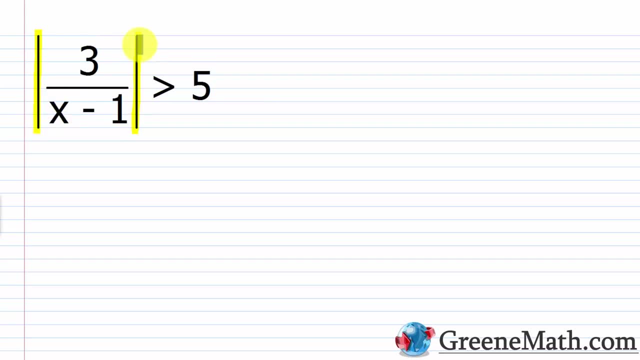 isolated for us on one side of the inequality. So you have this absolute value operation and this is greater than five. Okay, so for right now, don't even worry about what's inside of there. Just think about the fact that earlier in the lesson we said if we had the absolute value of x and this: 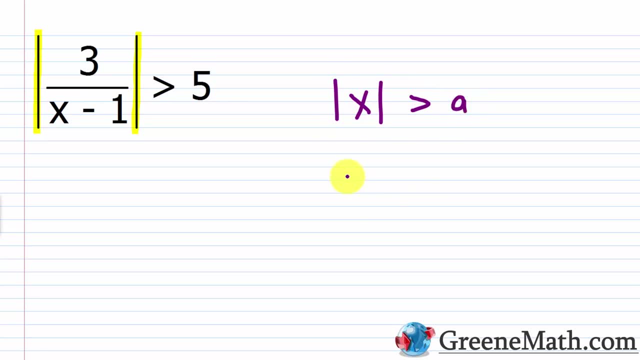 is greater than some positive real number, a. this led to x being greater than a or x is less than negative a right With our example. we said: if the absolute value of x was greater than seven, we said x was greater than seven or x was less than negative seven. Okay, so this should be pretty crystal clear at. 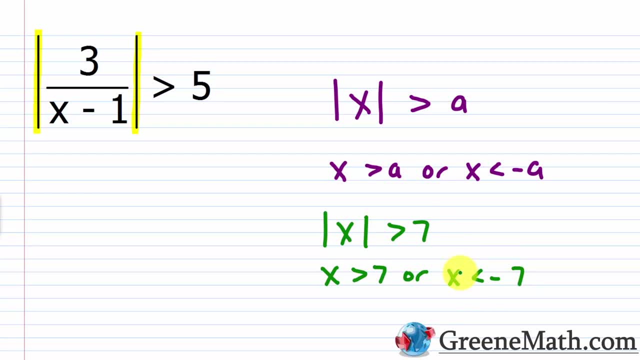 this point. Now, the thing is you can do this if you have a more complex expression inside of the absolute value bars. Okay, so I can replace this x with something generic like u. We'll just say u is some algebraic expression, So it could be a rational expression like we have here. It could. 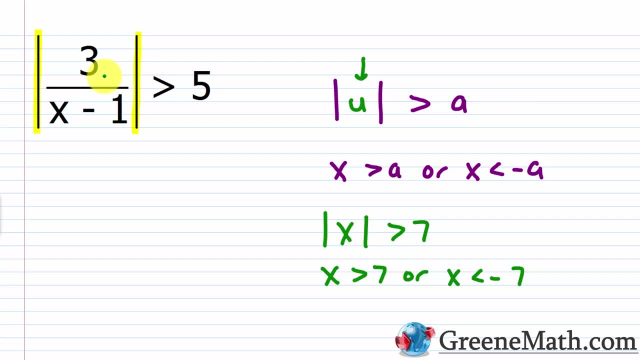 be a quadratic expression. It could be a quadratic expression. It could be a quadratic expression. It could be something more complicated than the typical linear expression that you're working with when you solve basic absolute value inequalities. So what I can do is erase this and erase the x. 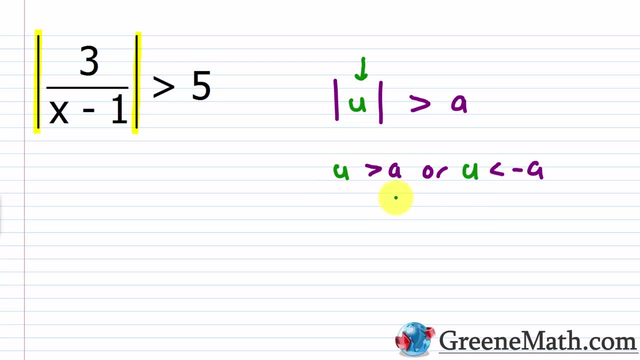 and just put a u there. Okay, so it's the same kind of concept, It just takes more time to solve it. It's just going to be way more tedious. Okay, so let's use this to set this up. So basically, 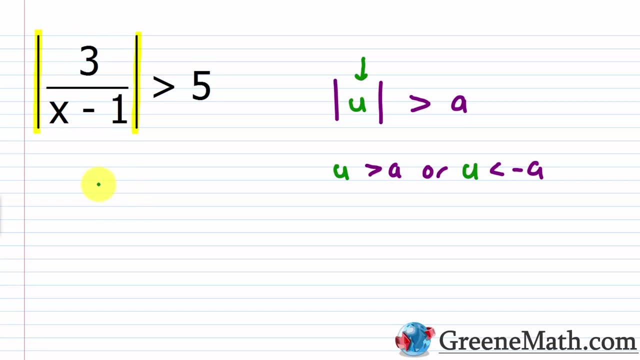 I'm going to take my rational expression inside the absolute value bars and I'm going to say three over x minus one. Since I have a greater than, I'm going to say it's greater than this positive number. five, then, or I'm going to say three over x minus one, I'm going to say, is less than the negative of. 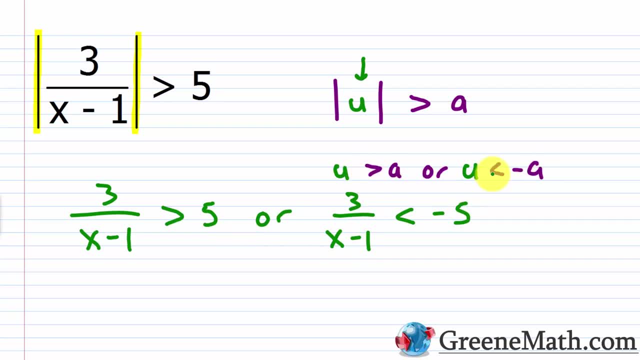 five. Okay, just use this rule here. That's all I did, Okay, so let me erase this. We don't need this anymore. So, basically, at this point, all we need to do is solve two rational inequalities and then kind of combine our two solution sets that we have. So I'm going to start out with 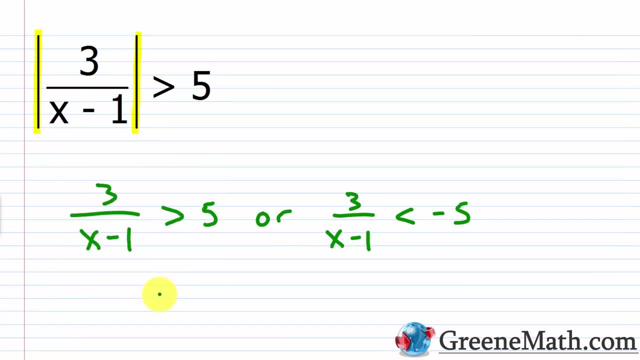 this one right here. So I'm going to copy this, we're going to copy this, and then I'm going to go down to a fresh sheet. Alright, so let me just paste this in here, And I want you to recall that. 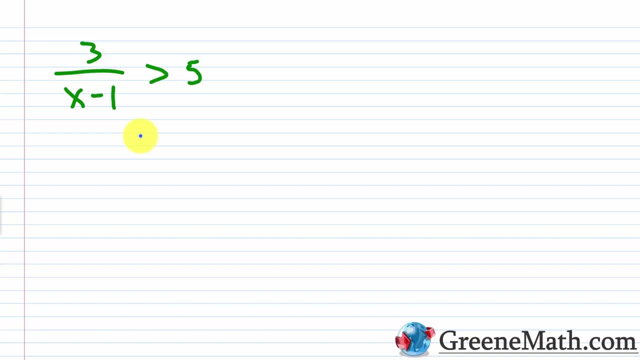 the very first thing you want to do when you're solving a rational inequality is get it in the format where you have a single rational expression on one side and zero on the other. Okay, so the way we're going to do that here is we're just going to subtract five away from each side of 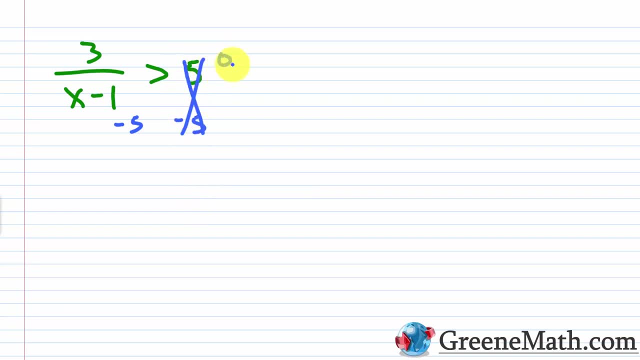 the inequality, And so this would cancel and become zero. So essentially I would have what I would have: three over x minus one, and then we'd have minus five and this is greater than zero. Okay, Now to get a common denominator going. let me just kind of slide this down a little bit, And what I'm 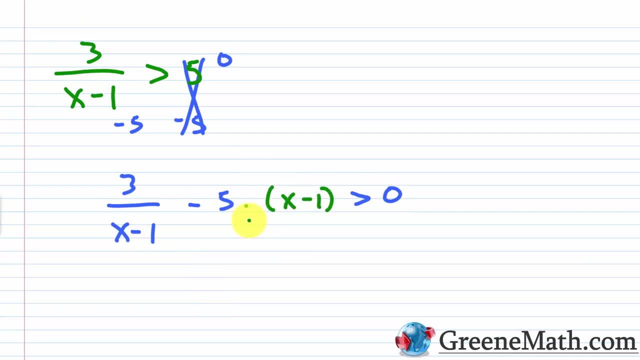 going to do is just multiply this by the quantity x minus one, and then over the quantity x minus one. So now I'll have a common denominator: negative five times x is negative five x, and then negative five times negative one is going to be plus five. Okay, So kind of continuing now I 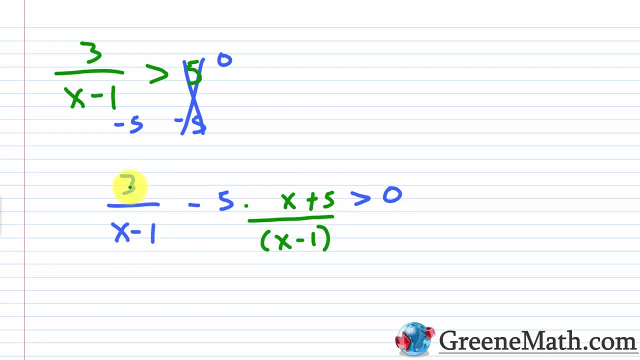 have a common denominator, So I can just combine the numerators. So we have three. and then- let me make this more clear- This is negative five x, And I'll just put a plus here. So we have three plus five, which is eight. okay, you have eight. and 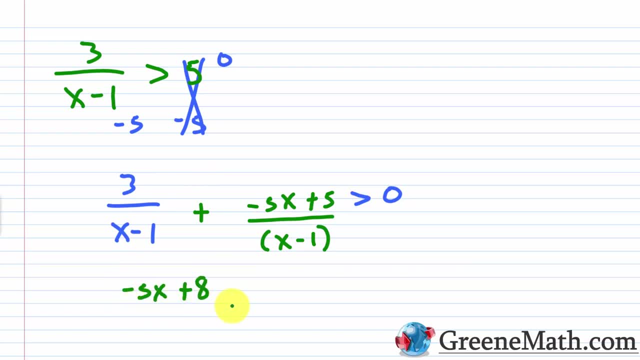 you have your negative five x, So let me write negative five x plus eight as the numerator. This is over the common denominator, which is x minus one, and this is greater than zero. Okay, so now we've accomplished kind of the first task. we have a single rational expression on the left side in: 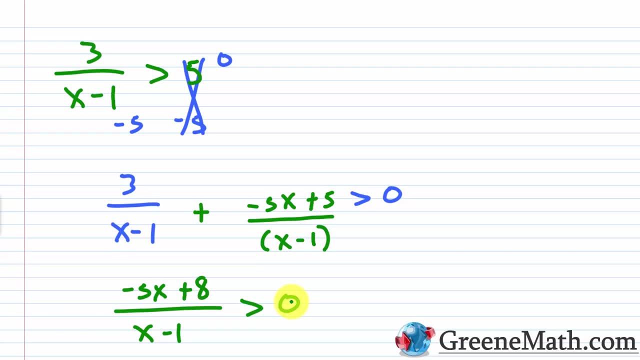 this case, and we have zero on the other. Okay, so the next thing we want to do is find out where the critical values are, or some people call them endpoints or boundaries, whatever you want to call them. okay, I'll just say critical values. So that is going to. 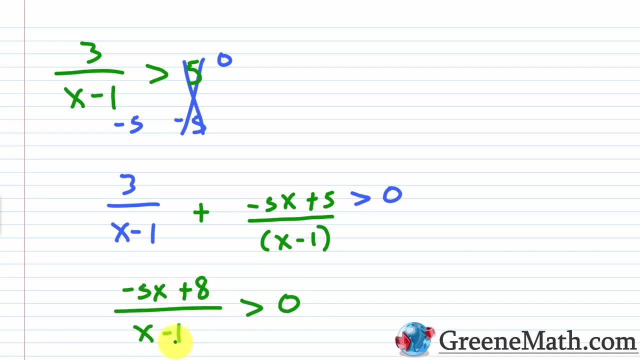 occur where the numerator is going to be zero and where the denominator is going to be zero. I would take this numerator, which in this case is negative- five x plus eight- and I would set it equal to zero. So that's one of them. then I would take the denominator which is x minus one, set that equal. 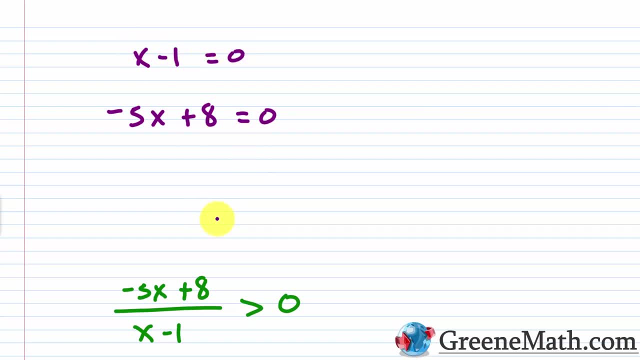 to zero. So both of those guys. when we solve that, the two solutions there are, the critical values- are again endpoints. So let me add one to both sides Of this equation that gives me x equals one. So that's one of those guys. let me subtract eight. 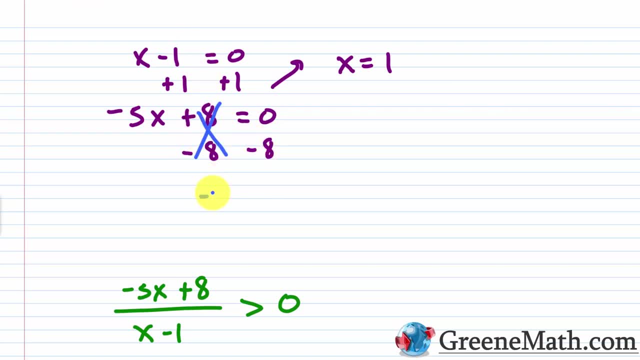 away from each side of this equation. this is going to cancel. you'll have negative five. x is equal to negative eight. divide both sides by negative five and you're going to get that x is equal to eight fifths. So these are our two critical values. So we're going to use that to 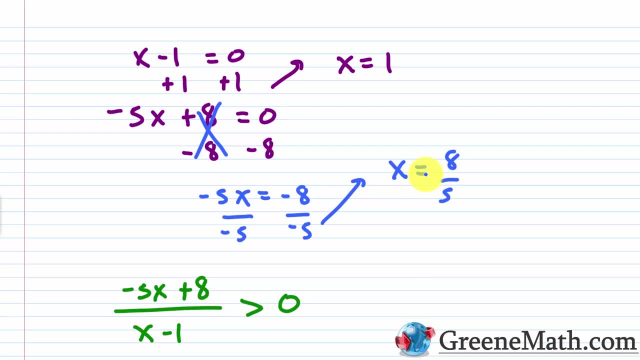 split the number line up into three intervals. So basically you'll have from negative infinity up to, but not including one, and then between one and eight fifths- right, neither is included- And then anything greater than eight fifths. Okay, so those are the three intervals you're going to. 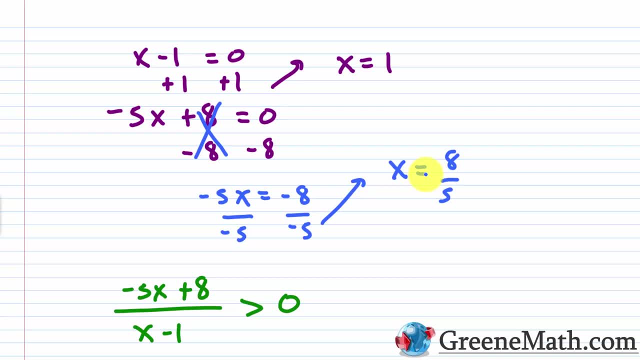 have. you're going to pick a number in each interval. okay, you're going to test that number in the original inequality. you're going to see if it satisfies it. if it does, that interval works. it's part of your solution set. If it doesn't, it gets rejected. it's not part of the solution set. 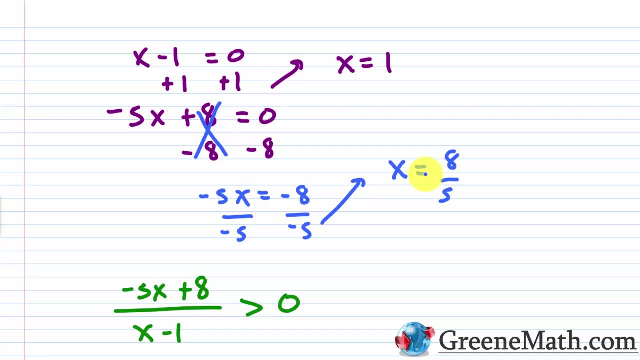 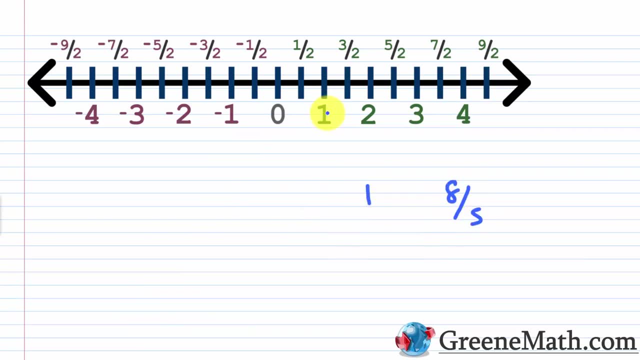 So you can use a table for this if you want, or you could do a number line For these. I prefer to actually use a number line, So let's do that. Alright. so the critical values. again, we have one and we have eight fifths, So one is right here, So let me just draw. 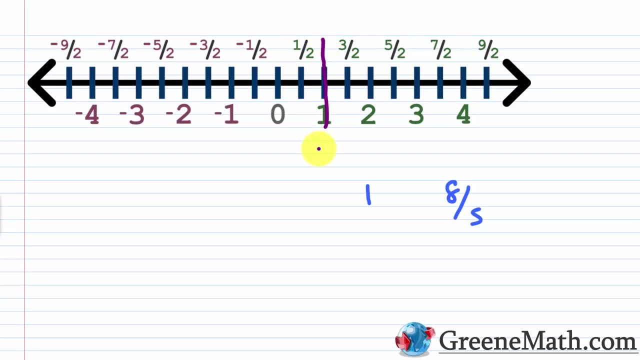 a nice little vertical line And it won't be perfect, but we'll put that in there. And then eight fifths is 1.6.. Now I've kind of divvied the number line up in a different way. you'll see that. 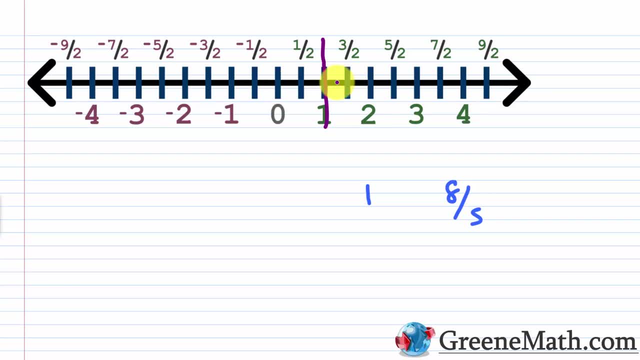 the notches here are separated by point. five or a half, So from one we go to 1.5, or you could say three halves, So eight fifths again is 1.6. If this is 1.5, 1.6, let's just say it's about right. 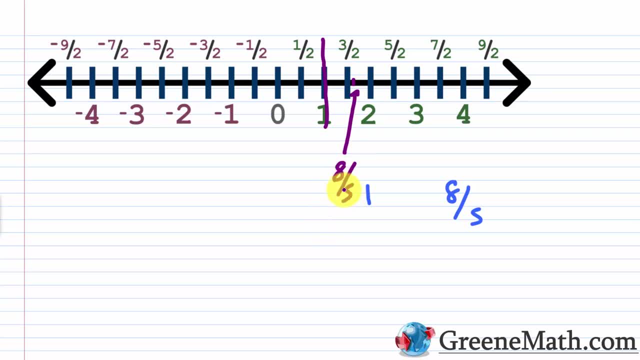 there. Let's say this is eight fifths. Okay, So let's go ahead and put another kind of vertical line there. We're going to divvy up the number line and just basically say that- let me kind of make that a little better. We'll say that this is interval A, basically anything. 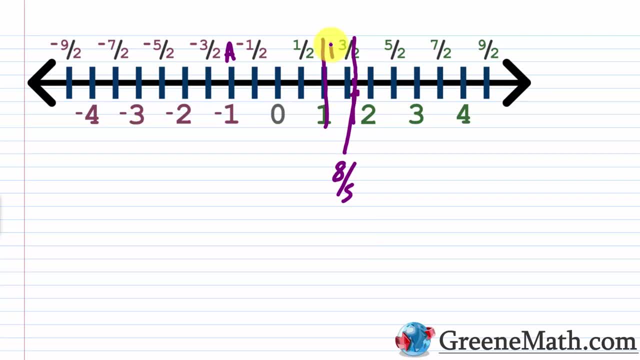 less than one, Anything between one and eight fifths, we'll call that interval B, And anything larger than eight fifths we'll call that interval C. So we'll have A, B and C. So the original inequality was three over X minus one is greater than five. So just take values in. 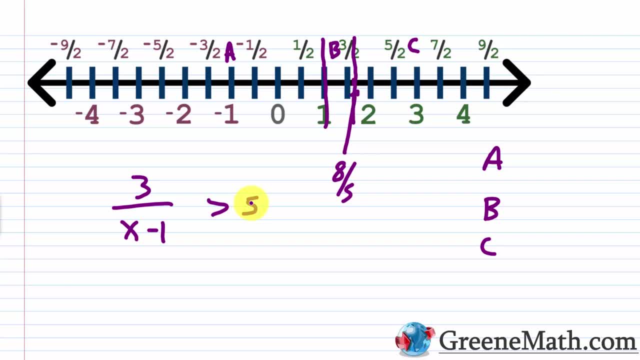 interval, check them see if they work Again. if they do, it's part of your solution, If they don't, it's not part of your solution. Very, very easy, Just a very tedious process. So from interval A I'm going to pick zero. Plug that in. there You would have three over zero minus one is negative. 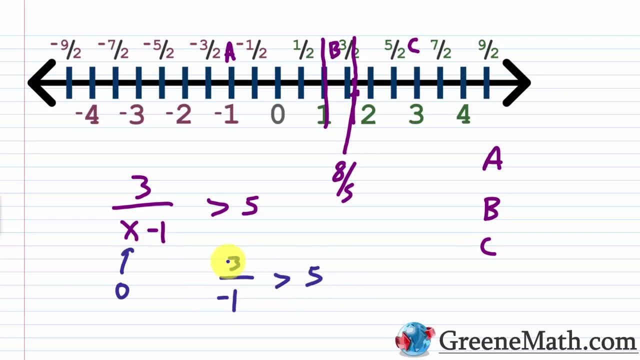 one, So three over negative one. Is that greater than five? No, This would end up being negative three. Negative three is certainly not greater than five. So this is false. right, In interval A, nothing's going to work. So for interval B again. 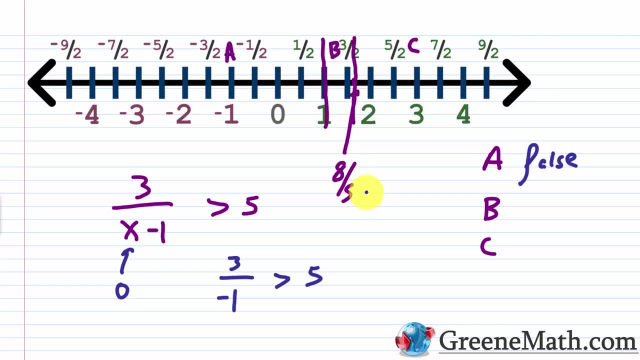 between one and eight fifths, or between one and 1.6, I think the easiest number to use there would be 1.5.. So let's go ahead and plug in a 1.5 there. 1.5 minus one would be 0.5.. So you. 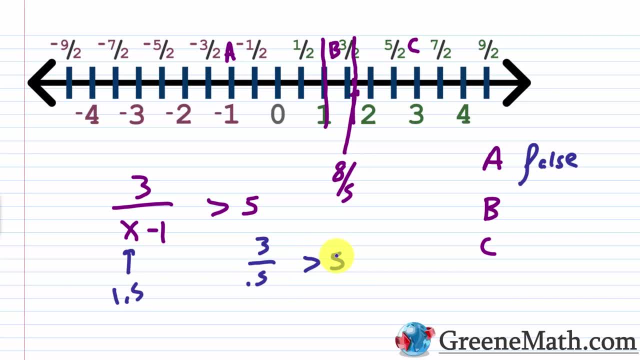 would have. three divided by 0.5 is greater than five. You know, if you divide three by 0.5, it's the same thing as multiplying three by two, right? If you divide three by a half, you could say: when you crank that out, you get three times two, which is going to be six. 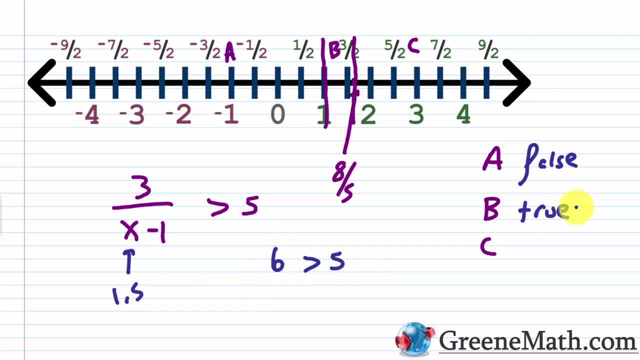 Is six larger than five? No, If you divide three by a half, you could say when you crank that out: yes, it is So this is true. All right, For the last one. let's take a look at something in. 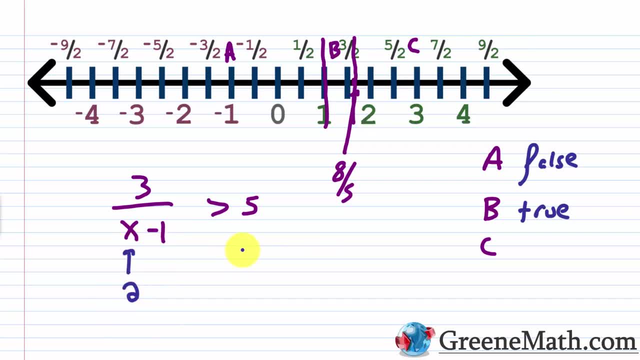 interval C, I'm going to pick two. So two minus one is one. Three over one is three. So you basically have that three is greater than five, which is false. Okay, Let me write that a little better. So false, Okay. So only numbers or only values in interval B are going to satisfy this. 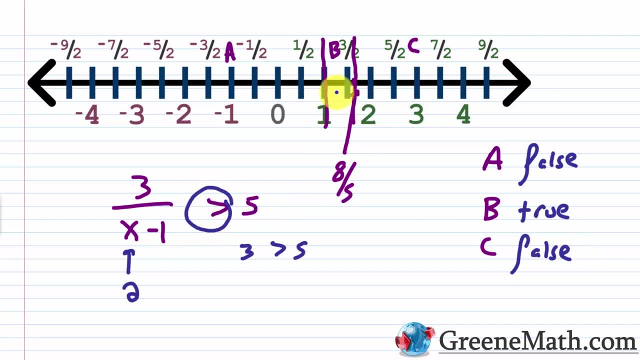 inequality. It's a strict inequality, So the end points we don't even need to consider. Okay, They won't work, They will be excluded. So the solution for this part is going to be anything larger than one up to, but not including eight fifths. So let's just copy this and we'll go back up And 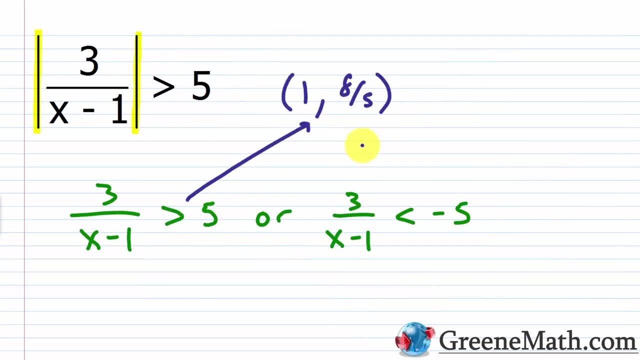 again, this is just going to be a partial solution. So this is for this one, And we could really write that X is greater than one and it's less than eight fifths. Okay, So this is just a partial solution. We're going to work on this guy now and see what else we can find. 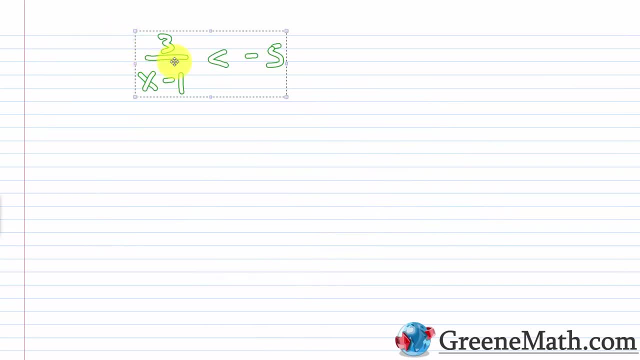 So let's copy this and let's go down. All right, So let's paste this other scenario here: We have three over X minus one, and this is less than negative five. So again I want to get one rational expression on one side, or one fraction, and zero on the other. So same process as last. 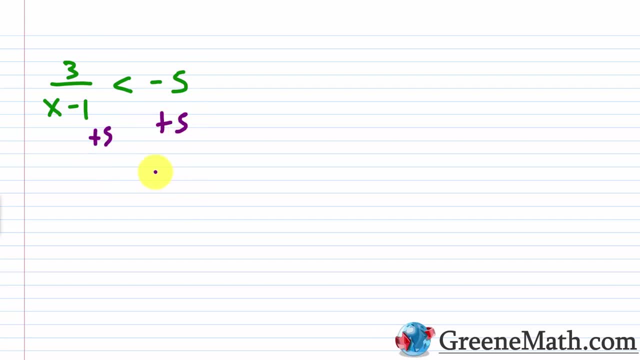 time. So I'm going to add five to both sides of inequality. I'm going to have that three over X minus one. then plus five is less than zero. I'm going to get a common denominator. So let me again write down. So I'm going to multiply this by X minus one over X minus one, And this is going to 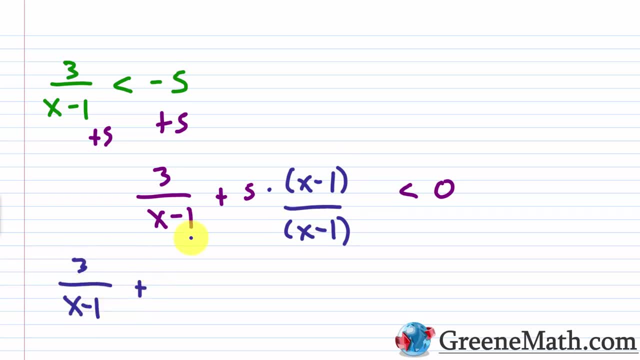 lead to three over X minus one. Plus, you have five times X, which is five X, and then minus five times one is five, And this is over X minus one. Okay, Then this is less than zero. So let me erase this. 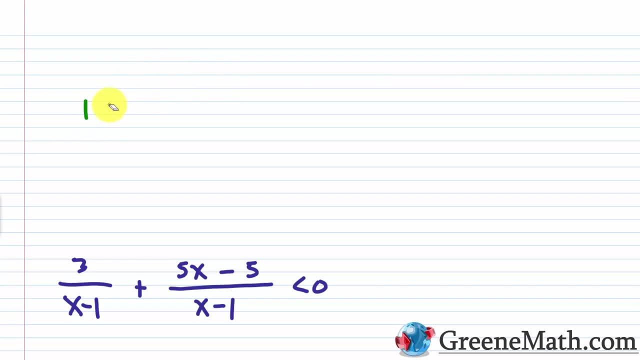 and we don't need this for right now. We'll write it again when we need it. So let me just drag this up and we'll make that three Little bit better. Okay, So now we're just going to kind of combine the numerators. We have a common 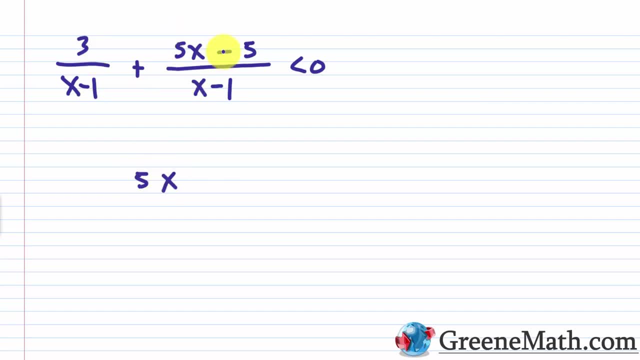 denominator. So we'd have five, X, and then three minus five is negative two. So minus two. this is over X minus one and this is less than zero. Okay, So at this point again, I want to take my numerator, set it equal to zero. take my denominator, set it equal to zero. That will give me the two. 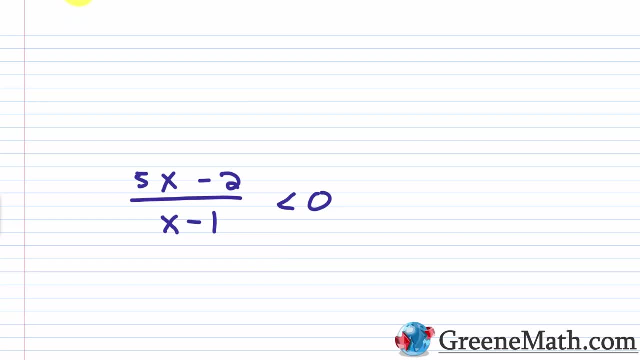 end points or critical values or boundaries. Okay, So we would have: five X minus two is equal to zero, and add two to both sides of the equation, I'm going to get that five X is equal to two. We would divide both sides by five and find that X is equal to two fifths. Okay, So that's one critical value And then X minus one. 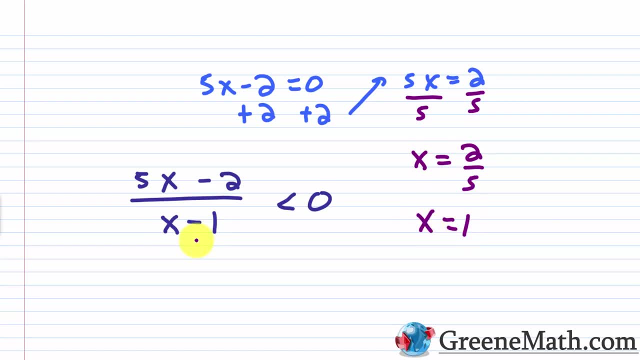 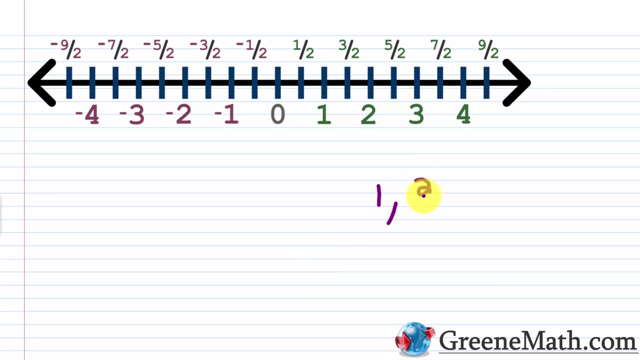 we know, if we set that equal to zero, we would get that X equals one. right, We solved that earlier. Okay, So let's go up And again the two critical values. we have one, and then we have two fifths. Okay, So one is right here. Let's. 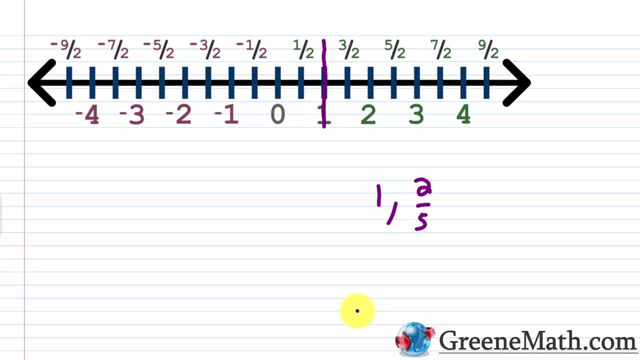 just put a vertical line there. Two fifths in decimal form is 0.4.. So I have a notch for one half 0.4 would be just a little bit less, So let's just say it's right there. So this is going to be my two fifths. Let me just put. 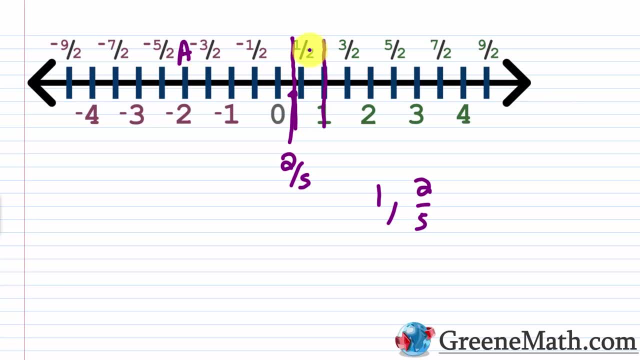 a vertical line there. Okay, So we have interval A, interval B and interval C. Again, interval A, in this case, is going to be anything that's less than two fifths, Interval B will be between two fifths and one, and interval C will be anything larger than one. So the inequality we're working. 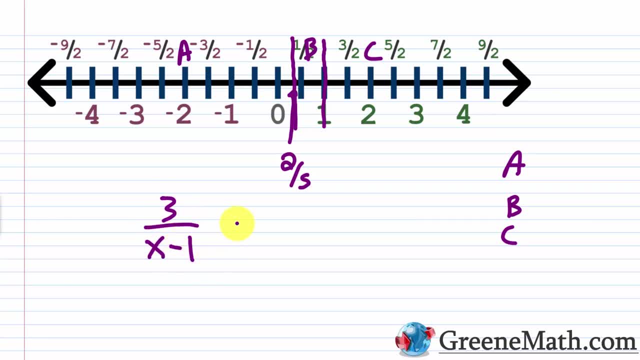 with is three and a half, So we have a notch for one half. So we have a notch for one half, And here we have a three over x minus one, and that's less than negative five. So let's choose a number from. 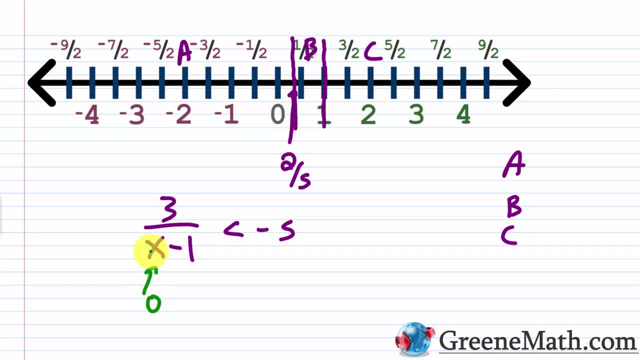 interval A: Again, I'm going to choose zero because it's easy to work with. So zero minus one is negative one. You would have that three over negative. one is less than negative five. That's going to be false, right? This would be negative. three is less than negative five: Negative three. 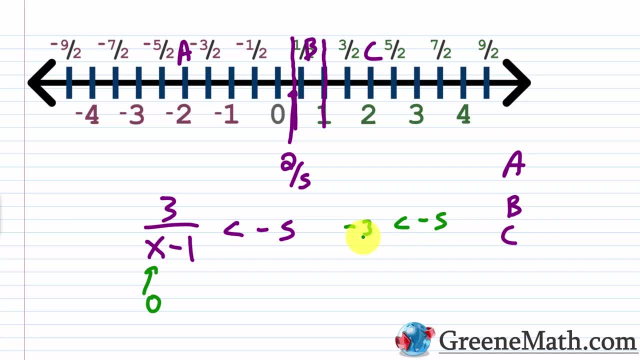 is a smaller negative value than negative five, So it's actually a larger number, right? So this is going to be false, Okay? What about for interval B? Well, it's kind of a tight window, but between two fifths and one. 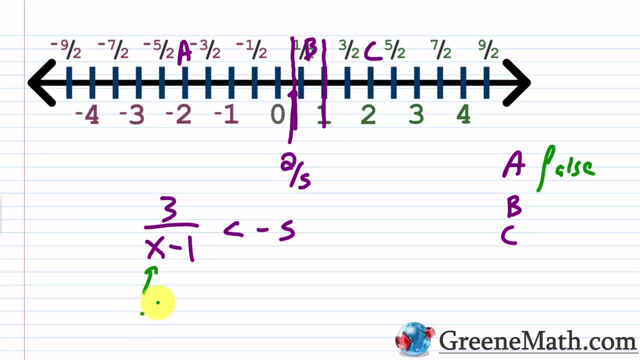 you can use one half. So if I do 0.5 there, I'm going to have 0.5 minus one, which is negative 0.5. So I would have three over a negative 0.5, and this is less than negative five, Of course. 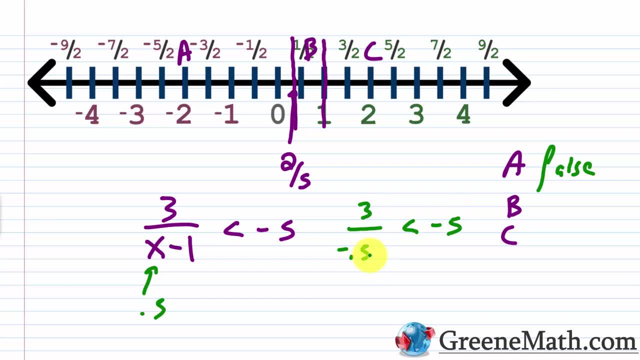 if I divide three by negative 0.5, it's like multiplying three times negative two. So this would basically be negative six. here Negative six is a larger number than negative five, So it is less than negative five. So this is true. Then for interval C again, I'm just going to 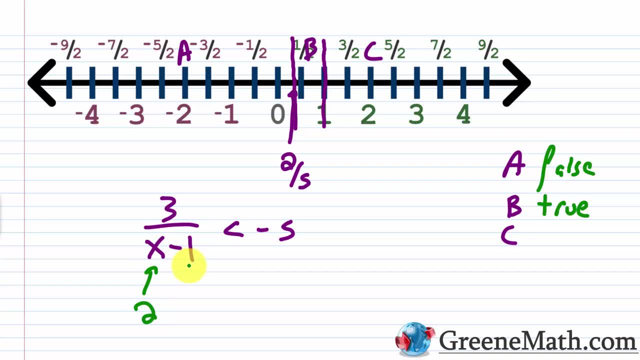 choose two, Nice and easy to work with. Two minus one gives me one, So I would have that. three is less than negative five, which is obviously false. Okay, So my solution here is going to be, for interval B, anything between two fifths and one. So between two fifths and one. Okay, So for this. 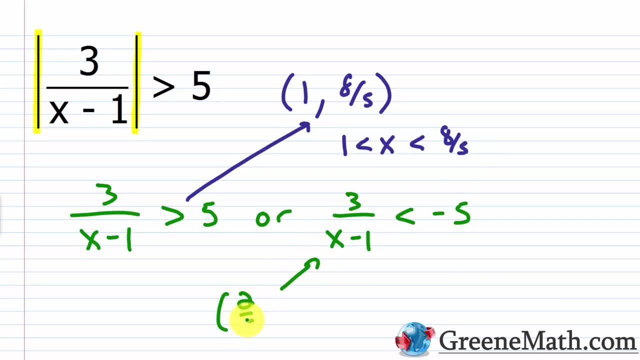 guy. my solution is again between two fifths and one. So now I'm going to have two over a negative five. Now it's going to be the union of these two solution sets. So let me erase this. I don't need. 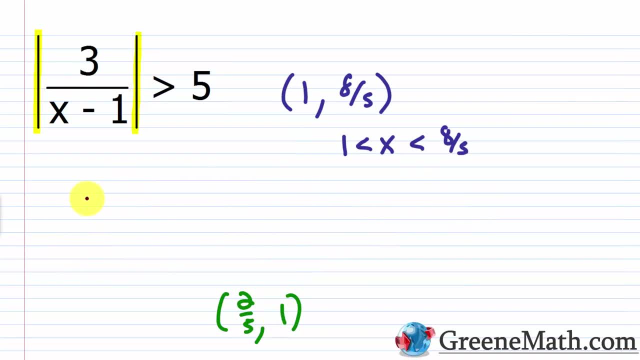 any of this anymore, because I'm thinking about the problem as a whole now. So I'm just going to start with this one. So I'm going to say between two fifths and one. again, neither is included. And the union with this guy, which is between one and eight fifths, neither is included. Okay, Now you.